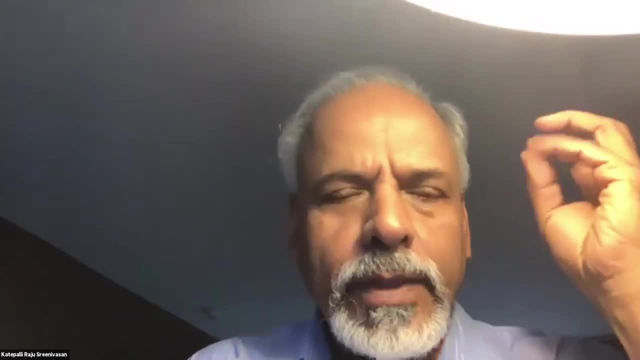 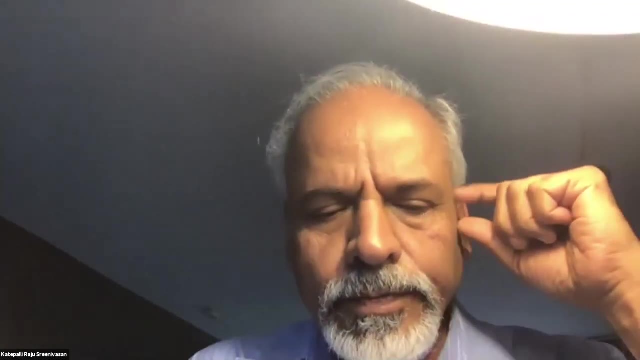 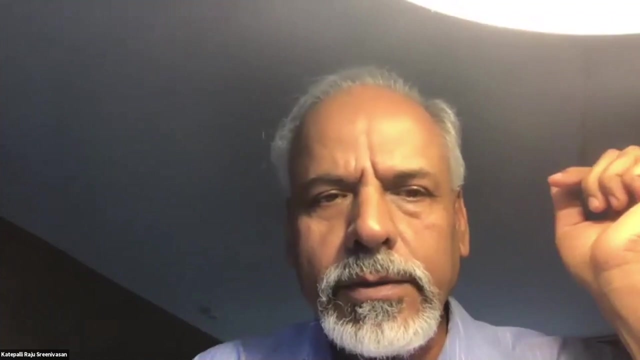 I look forward to the talk very much. At another time. I hope when the situation improves, we can have you back in NYU Abu Dhabi physically. So I want to welcome all of you to this webinar And I will now hand it over to Demetra to say a few words about the speaker or anything else. 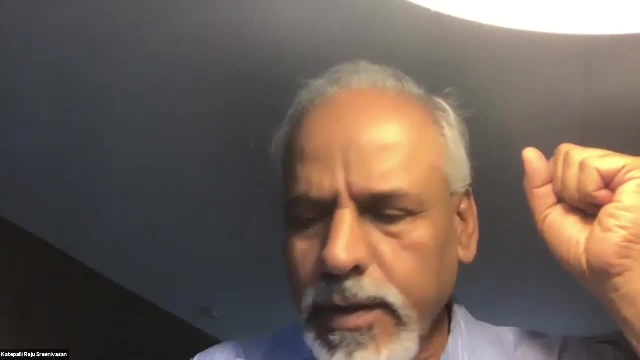 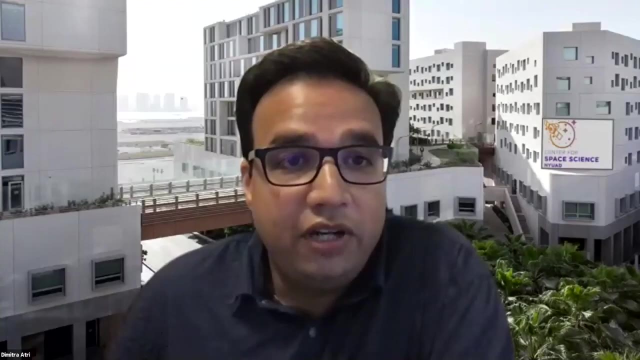 he wants to. before we let the speaker give us his talk, Thank you very much again for joining this. Yeah, thank you, Srini. Can you hear me? Srini Srinivasan PhD. Yes, I can hear you. 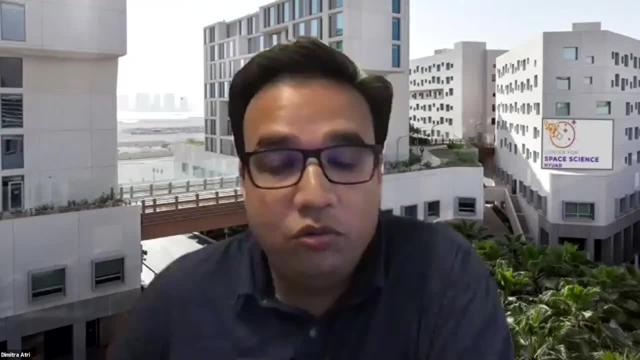 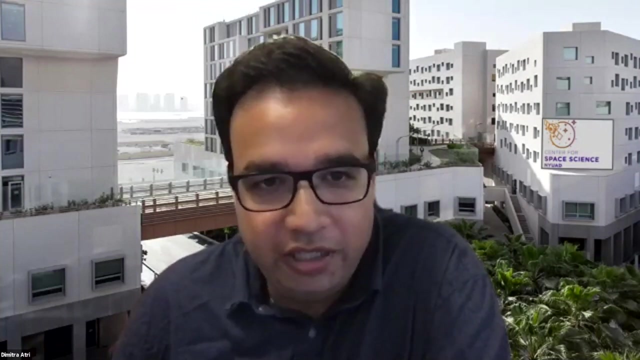 Well, I can, Yeah, Demetra Dugas- Okay, cool, Great Yeah. So welcome everyone. Thanks, Srini, for the nice introduction, So welcome everyone. Good morning, good afternoon, good evening, wherever you guys are, Welcome to the Space Science Webinar Series in collaboration. 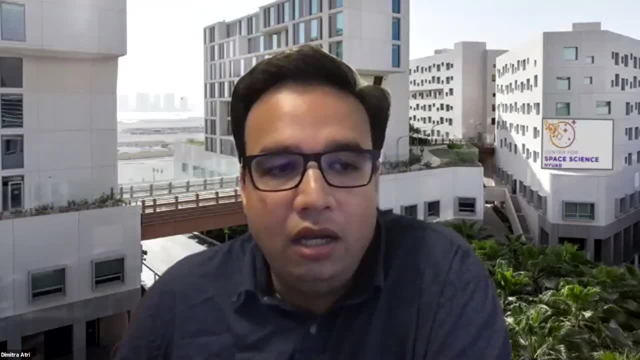 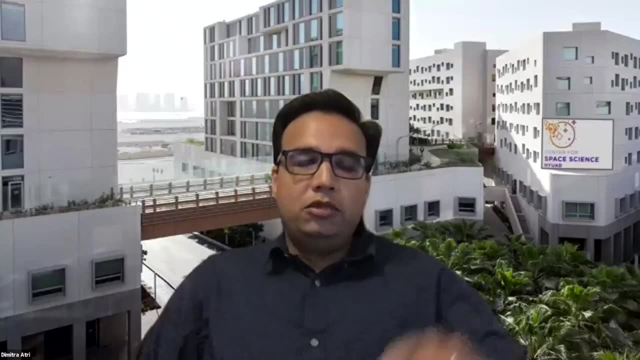 with the UAE Space Agency. So this is a weekly seminar every Tuesday at 3 pm. GST- Demetra Dugas- So just below you can see this chat feature. So feel free to use that feature for discussions amongst all the participants. If you want to message somebody individually, you can do that. 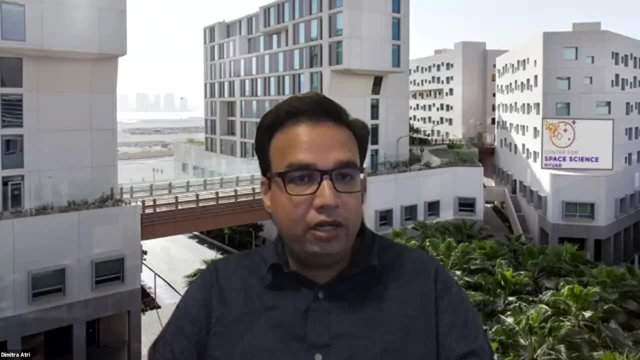 You can also ask any questions to the panelists. There is also a Q&A section which you can see below. You can use the Q&A feature to ask any question to the speaker, But I would recommend you doing that towards the end of the talk. Demetra Dugas- Okay, thank you very much. 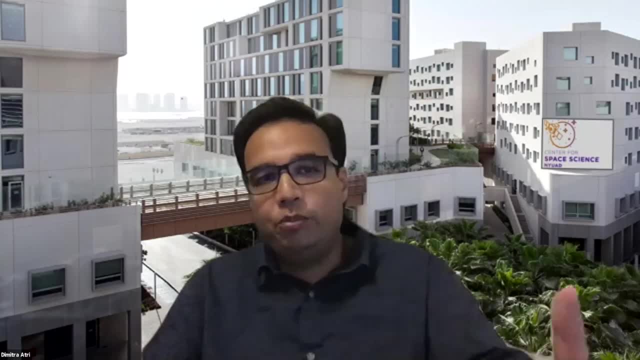 everyone. Thank you, Demetra Dugas-. So we will now go to the Q&A part of this webinar, because otherwise it is really difficult on a computer to stop everything, read the question and then respond. So after the talk I have like 10, 15 minutes. 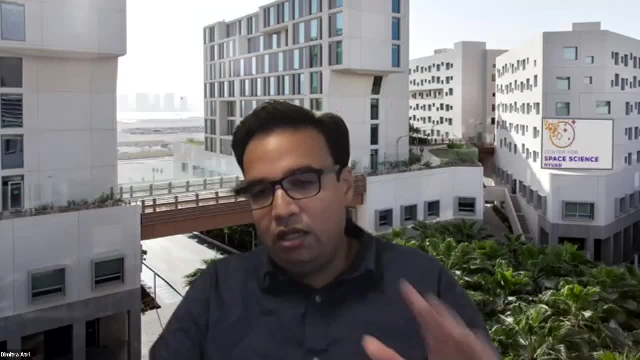 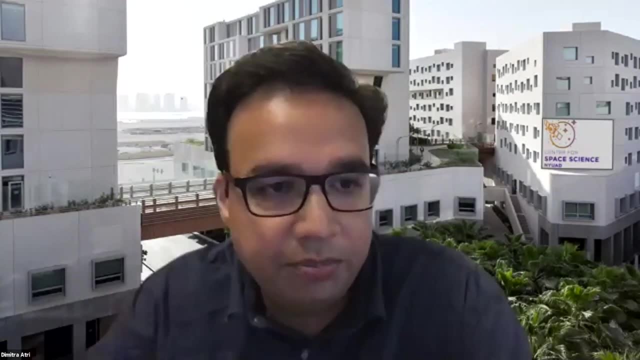 You can post your questions then, and then we will go through them one by one. We can even, at the end, ask you to turn on your microphone and have the question asked you directly, recording this, and we will be uploading this somewhere, probably on YouTube. 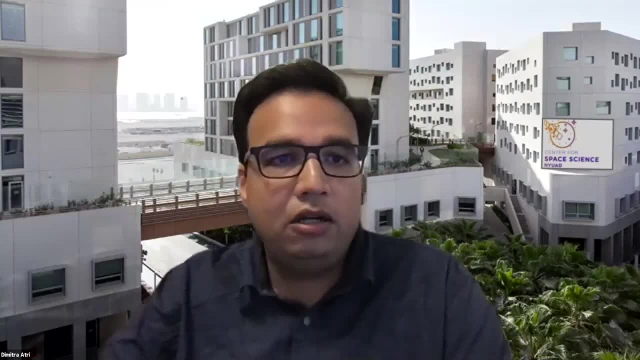 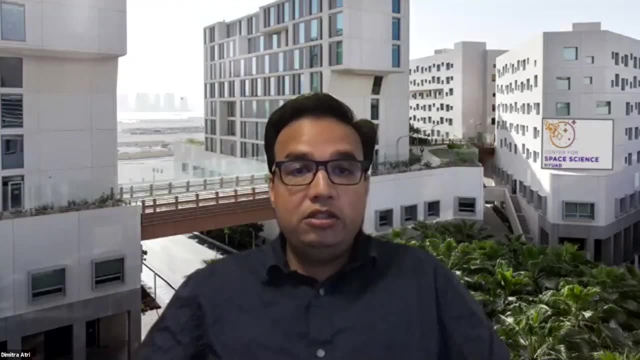 Other than that, all the whatever chat, all the transcripts are also going to be recorded. Once again, I thank the UAE Space Agency for doing this, collaborating with us. So to get started, let me introduce Dr Guillaume Grunoff for being our first speaker. 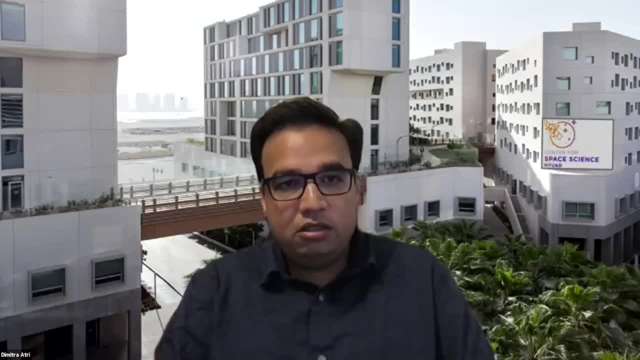 I have known him through his numerous publications. He's a well-known expert in the field. He got his PhD from Joseph Fourier University in Grenoble, France, in 2009.. After that he moved to the US. He started as a postdoc at NASA Langley Research Center in Virginia and has been a professor. 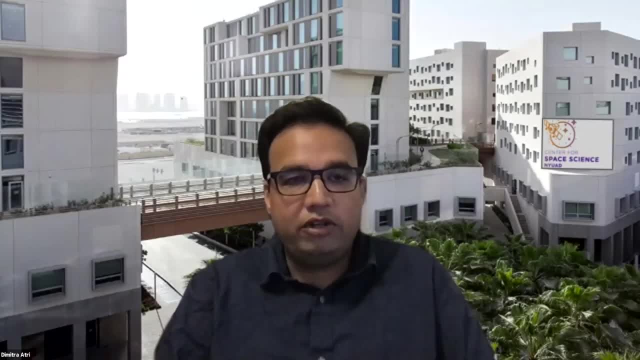 there ever, since He has a very large body of work on how radiation interacts with planetary atmospheres. So thank you, Guillaume, for agreeing to do this at 7 o'clock in the morning for us on the East Coast. Yeah, go ahead. 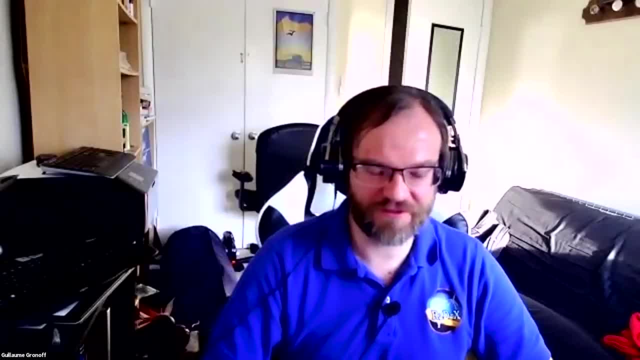 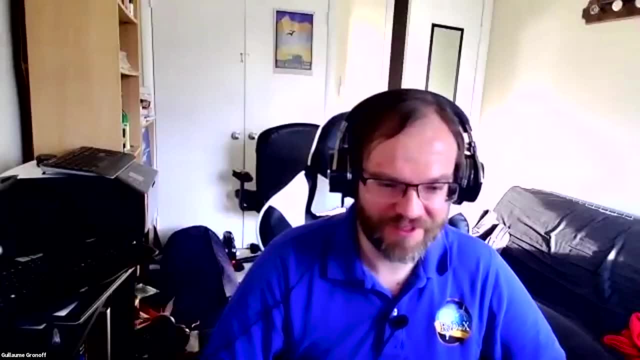 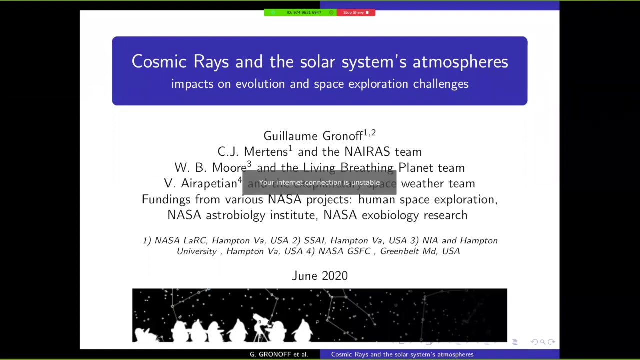 Guillaume Grunoff. Okay, but thank you very much for inviting me. It's a great honor to be able to speak to you, Thank you. I will go and speak a little bit about my work on cosmic rays and on the solar system's. 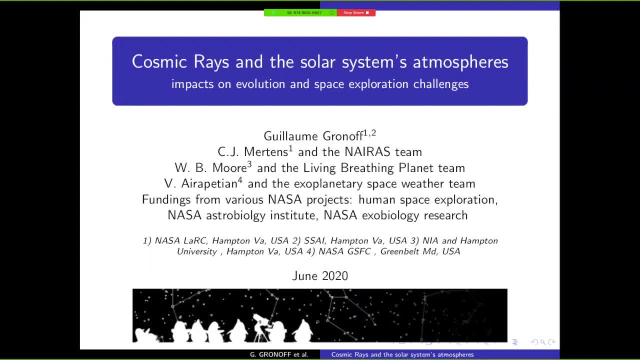 atmosphere, the impact of the system and atmosphere, and really it's speaking about all what this cosmic ray do in the solar system, Thank you. So what the solar system right now did in the evolution of the solar system and what has the evolution the impact for the space exploration? what are the challenges for the 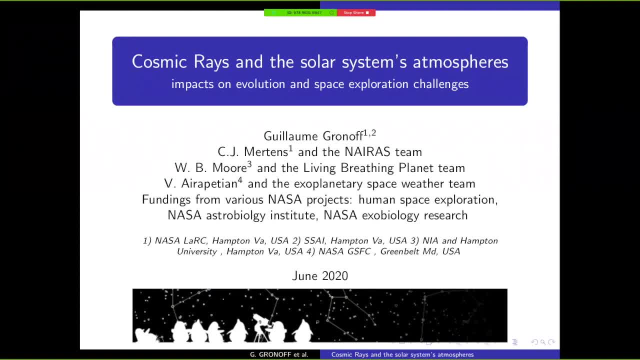 space exploration. So that's a large part of the work, but I'm really doing this to explain the whole breadth of what the cosmic ray problematic is for us. So I cannot do that seminar without thanking all my collaborators, friends and co-authors. 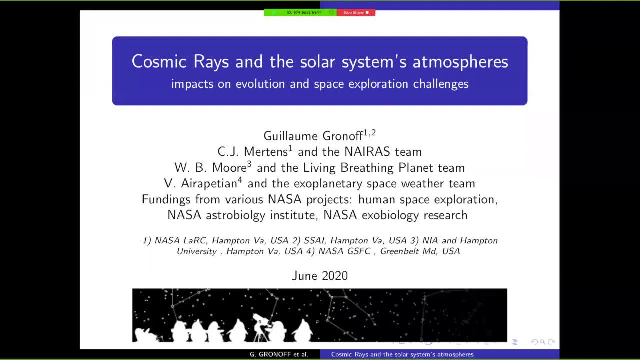 on the different projects that I have been working on for this presentation. There is not enough space in this slide and actually in the whole presentation, So I'm going to give you a little bit more time. So I'm going to give you a little bit more time. 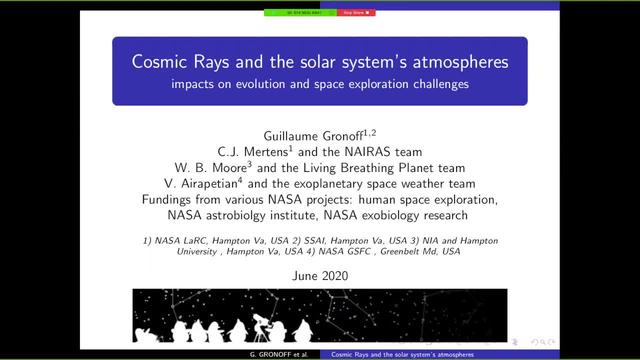 So I'm going to give you a little bit more time. So that's the whole presentation to list everybody. So I'm sorry for if you don't see your name and if you have worked with me, I'm just putting a little bit of the people and the funds, people who funded me. so the different team. 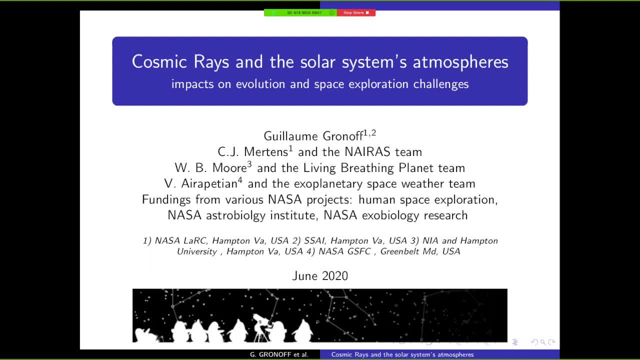 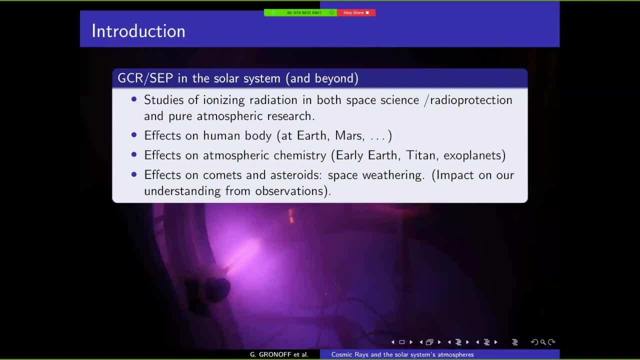 but everybody is extremely important for this work, Thank you. So let's start Here. we are going to speak about the GCR and SEP. So when I say that GCR, SEP, everybody says it like that. It's Galactic Cosmic Ray and Solar Energetic Particular. 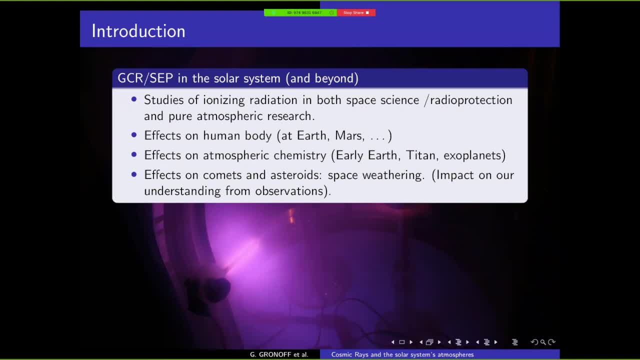 Event That's very important in the solar system and beyond because it's very energetic ionizing radiation. They have impact in radio protection problems. So for typically for astronauts, we think a lot about the problem of radio protection, But it's not only that. 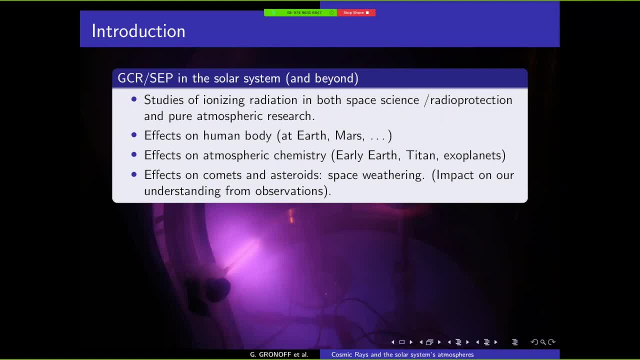 Even for the instrumentation. it's very important to have a good idea of how to protect this instrument in a very high ionizing radiation environment. And one of the point people are really thinking about there it's instrument flying near Jupiter. You have a large radiation belt over there and they can be very dangerous for the instrumentation. 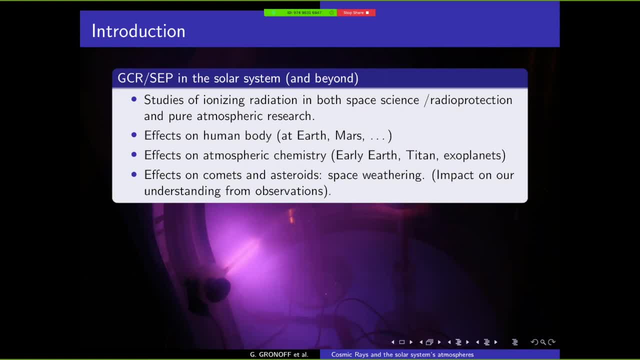 In addition to the effect on people and instrument, you also have effect on the atmospheric chemistry and you have effect on the bodies in themselves. We will see a little bit of that and a little bit of the questions that this has been asked, But just so that we have an idea we are going. 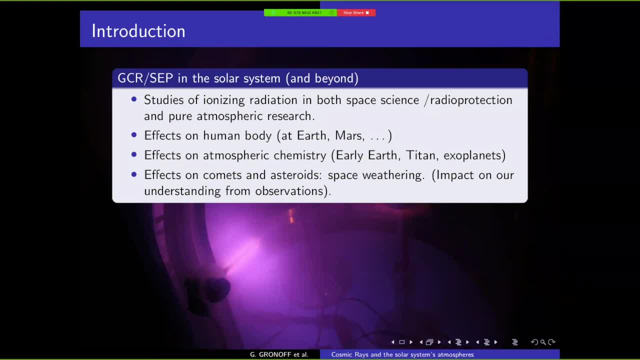 to start. So let's start, So, let's start. So when you start having ionizing radiation, you do some chemistry, You start creating a larger molecule, like in Titan, and you start to create some new compounds that can have a really big effect on the chemistry in itself And that can have feedback on the atmosphere. 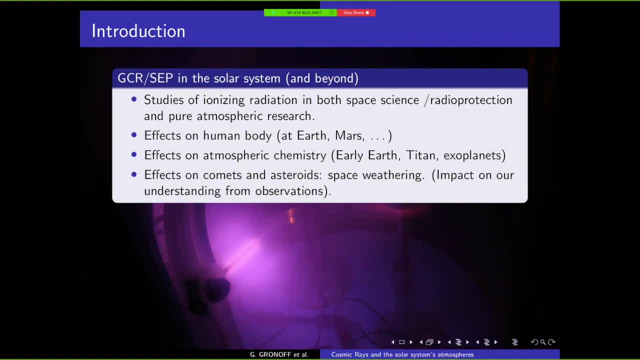 and its evolution. Finally, when we start to put this cosmic ray on asteroids, you can redo some space feathering, You can have a change in the exterior of the body And if you use a space mission to look at the exterior of the body, 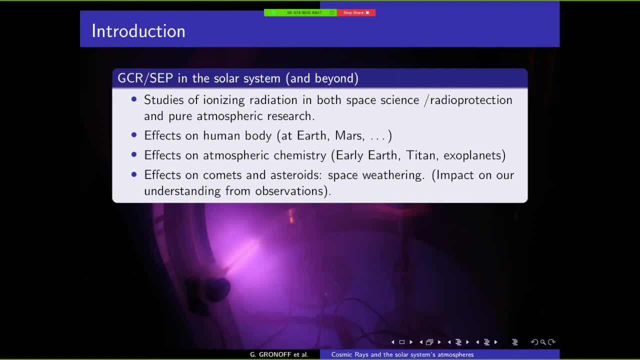 you will have. you won't have an idea of what the pristine object is, but you will see what the object that has been affected by the radiation looks like And you have to take that into account when you want to use this observation, for example, to infer what was at the beginning. 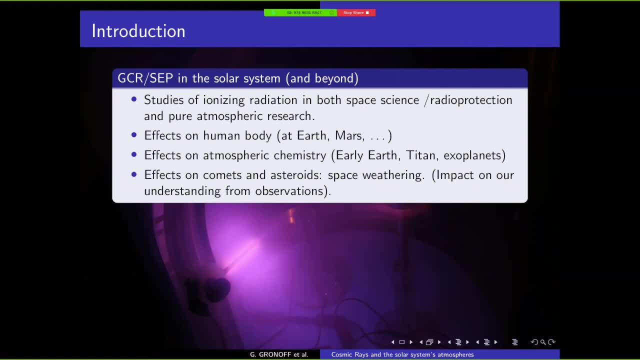 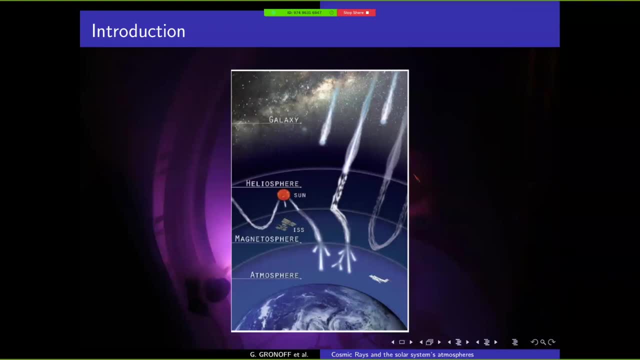 of the solar system. So to go back, and when I say SCP and GCR, I like that little presentation where you see the particle coming from the galaxy that are hitting the highest field, What they hit, the highest part of the elliot sphere, And sometimes, when they go into the 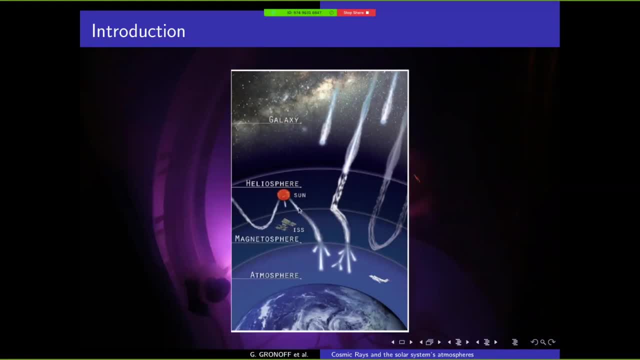 elliot sphere. they are pushed back away from the Earth, off planets. As you事情, you have the sun that suns its own particles, so energetic particle and most of the times, the most important part of the sun's very energetic 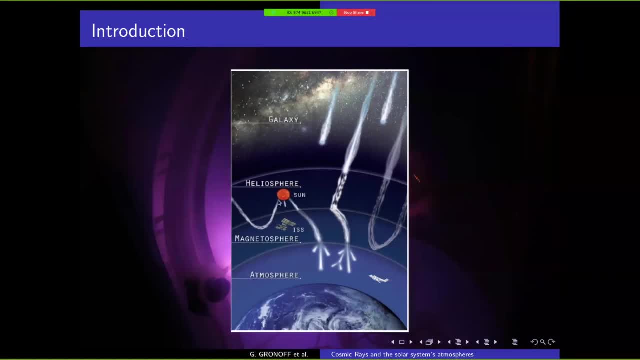 particle comes from the solar energy particles, so SEP events. so it's more with the storms and not something that is continuous like what we have with the galactic cosmic ray. Then when you come near the Earth you have the magnetosphere that prevents. 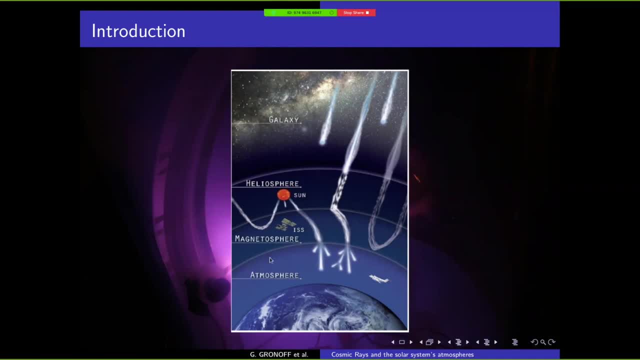 some of the less energetic of this particle to go lower, and we'll see that a little bit more later. And then you have the atmosphere and you have all the effect and most of the interaction between the cosmic rays and Earth are in the atmosphere. 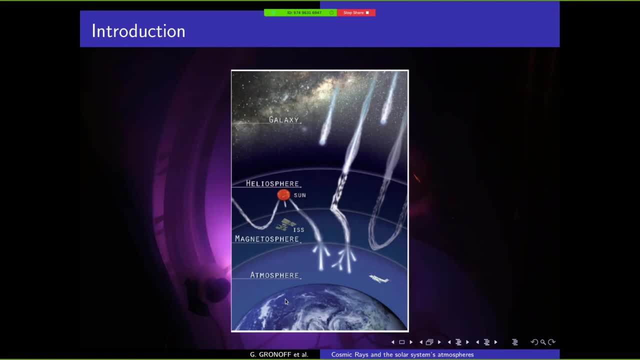 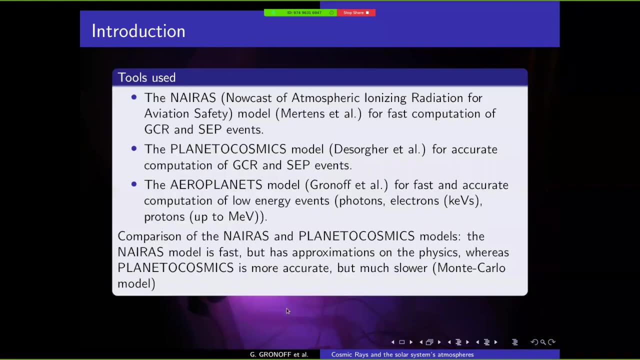 And typically the atmosphere, really protects Earth and prevents this particle to be at large quantity near the ground. So to study this, this effect of particles, I have several tools that I have been either developing or using or modifying over the past decade. 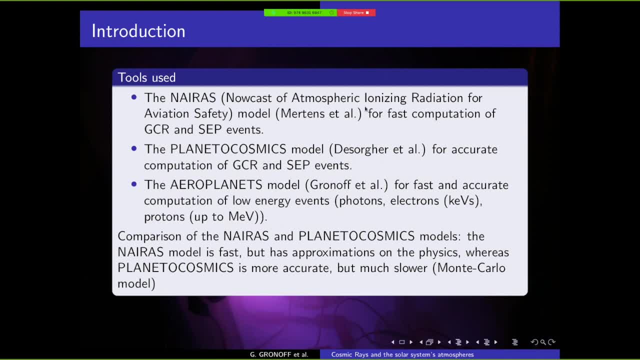 So you have NERAS, the knockout of atmosphere. I'm using radiation for aviation safety model, So it's a model for the fast computation of GCR and SEP event, with the idea to look at what happened on the Earth's atmosphere and to be able to say that if you take a plane, 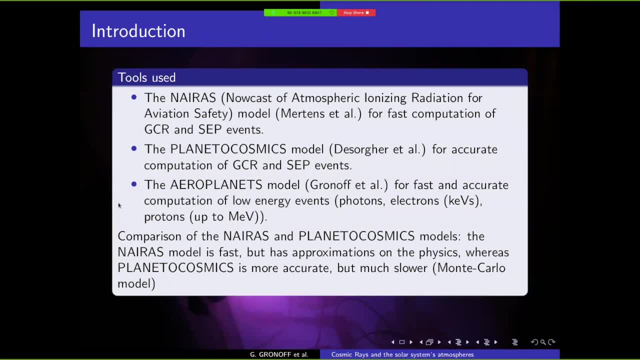 well, I hope we'll do soon. we will be able to. we have some radiation, more radiation, but we still have about one million particles on the body of the person when we go near the pole. So it's a problem because flight personnel is one of the group. 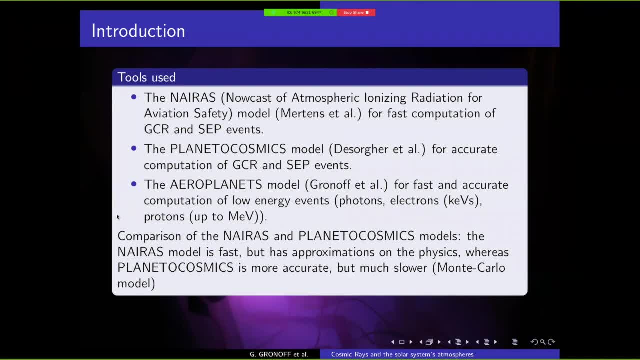 of people who receives more radiation per year And the most on. people work in nuclear power plants, So it's important to have a more reasonable amount of radiation. It's important to have a more reasonable amount of radiation, So there's a lot of energy and energy that we need. 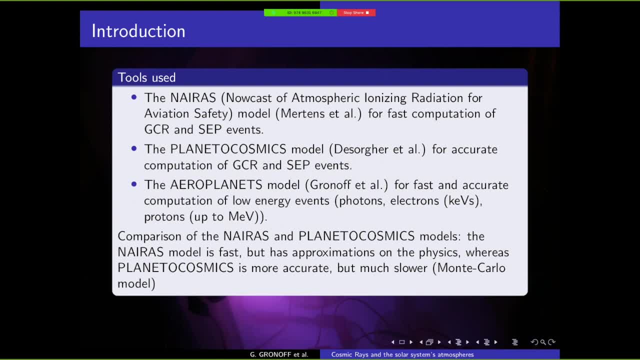 address how much radiation they get in terms of public safety. So that model is used for that, but has been also used for other kind of research and is being has been used for looking at Mars, for example. You have the planetocosmic model. That has been its a GenFOR based models. that has been really developed. 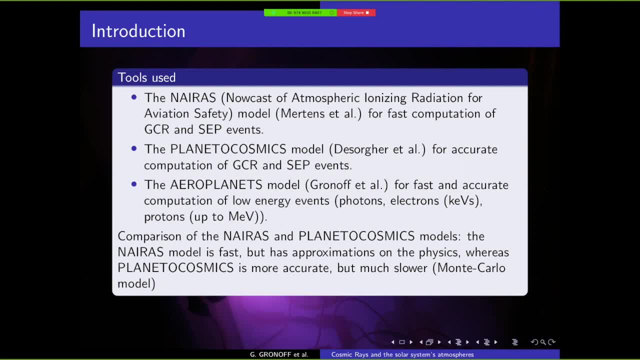 to look at the cosmic ray at all the planets. it's much more accurate and there has in Wish and Sab. we used much more physics in the model, but it's a Monte Carlo model so it takes a lot of time to run it and on top of, 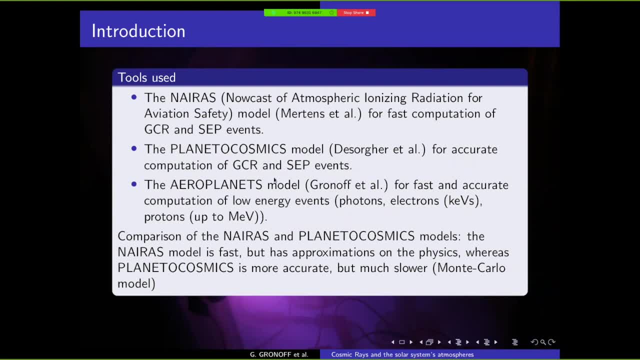 this model. I have my aeroplanets model that doesn't look like a cosmic ray and dissipate, but looks like at the lesser energetic particles or EUV, XUV, photons, electrons up to KeV, protons up to the MeV, and that allows to have a 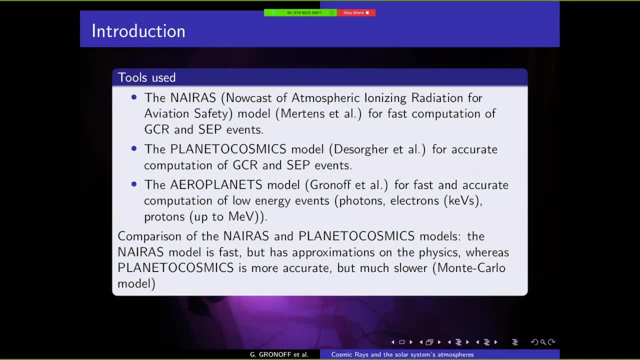 full picture of the ionization and it's really my contribution. my first contribution to the field was to put everything together to have a better idea of kinds of models and especially the NEA- sometimes paintocosmic- and compare them to be able to be sure that the faster model are. 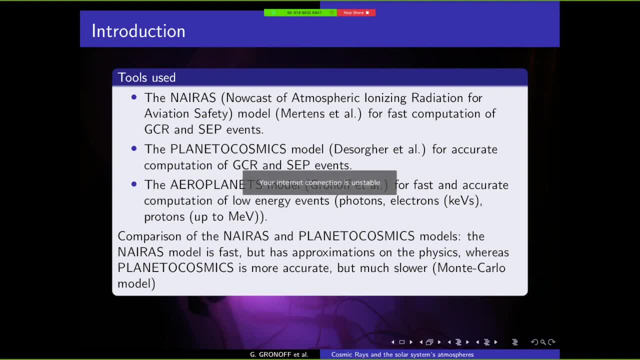 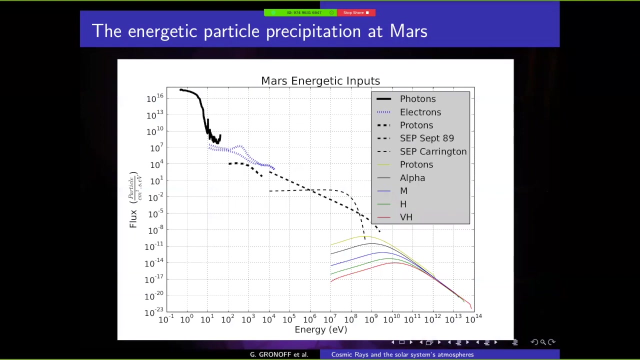 accurate enough to to give us a good vision of the radiation when we look at human impacts. So, speaking of human impacts of radiation now is: everything is more to Mars and of course it's. it's very important to to look at Mars with all the missions that go there and, of course, the UAE mission hope that will launch in a couple of weeks. 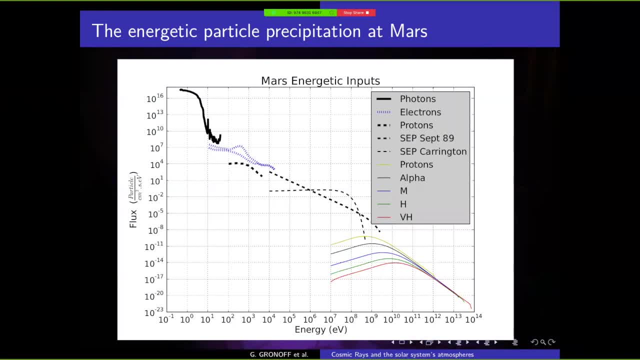 so that's a figure of of the energetic inputs at Mars. I like this. so on the top left we have all the photons from from the Sun, and when we start to be around them- sorry, around 1080- that's where we start to try nice, then we have the electrons, the blue and the blue and the orange, the organic electrons. so we have to get myself on that. damn, she's got a успion leave only about five minutes, but my him scream still got back at you. yellow, the blue, the blue. if you possible for me, mi, that's the, the rox, or or, and don't go over, I can see. 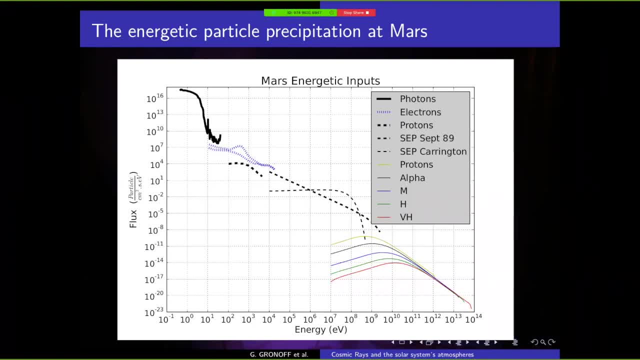 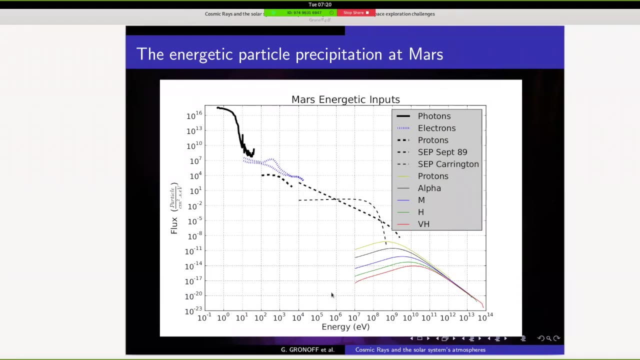 with you. let me call the blue and then, in the video I drop to youником, beyond the blue light, dotted blue, there is different spectra of this, of this electron, the precipitation, just because we have some. oh yeah, i was showing that. so, going back to the energy, the higher level of energy, 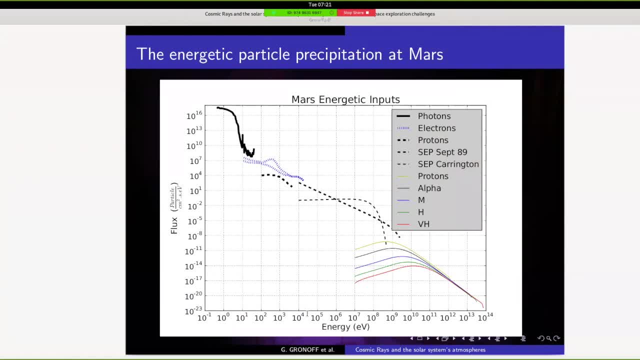 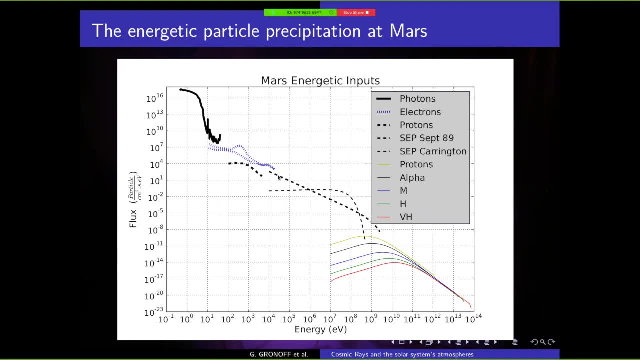 yes, like that. so now we start to go to the mev and that's where we start to see the, the very energetic particles and the events that start to be a to be strong. uh, so we have the scp events. so here it's. we have to be looking at that and saying that it's not what we Fra 빠. 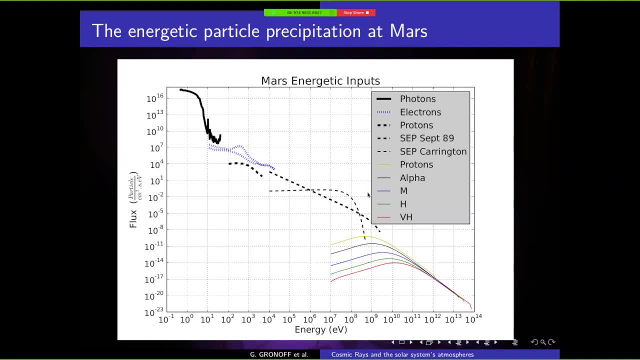 happen. normally That's a very energetic event and that's extremely rare, But they exist and that's something we can address. So typically you will have way less proton going into Mars, but in that case sometimes you will have big and strong cosmic ray event. 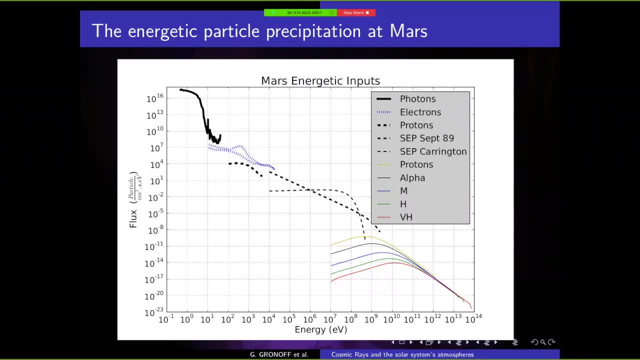 or SEP particle event and that would be dwarfing the cosmic rays at the gigaelectron volt. And finally the multicolored at the bottom right. it's all the cosmic rays. So I did show the cosmic rays only for a certain stellar activity. You have to realize that there is a little bit. 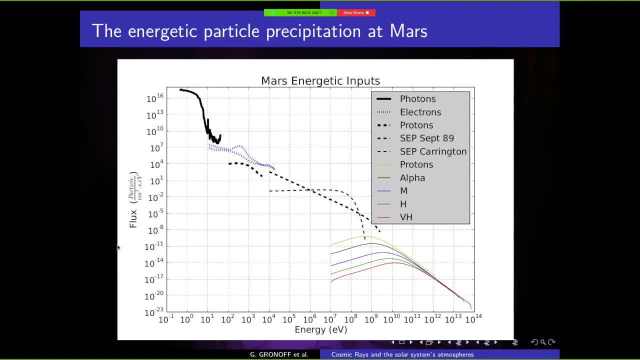 of variation of cosmic ray because the sun's heliosphere varies with the activity of the sun and that has an effect to shield the lower energy energetic cosmic ray. We'll see a figure a little bit more striking about that effect later. And I did put proton, alpha and the different MH and BH. It's a group of more energetic particles. 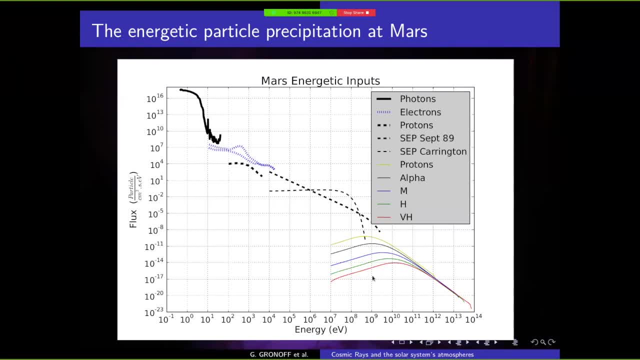 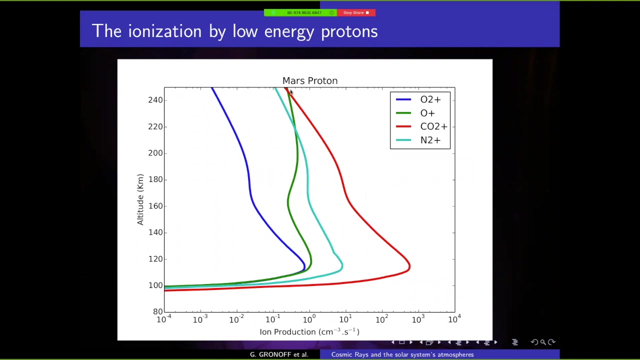 For example, you have to realize that BH is iron and even if there's fewer of it, because the particle is more massive, it gives a lot of energy and it has impact at different altitudes. So now we look at an example of computation. You have, for example, low-energy protons that can 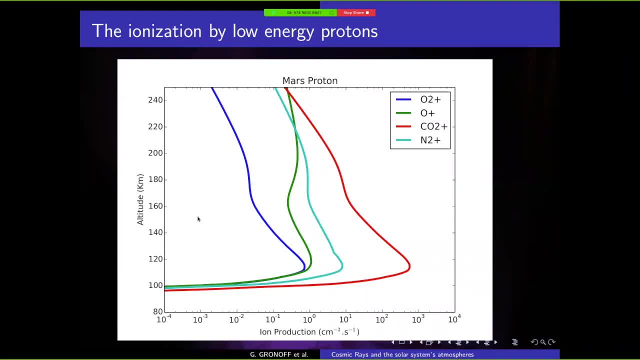 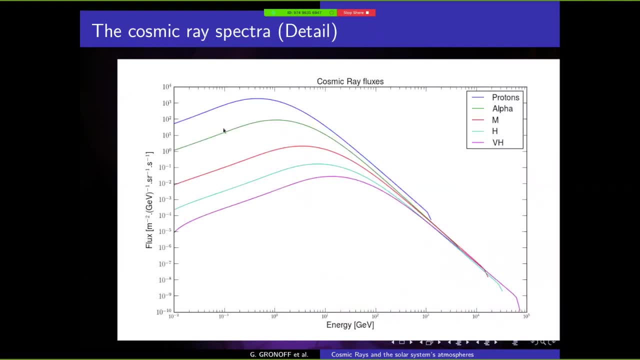 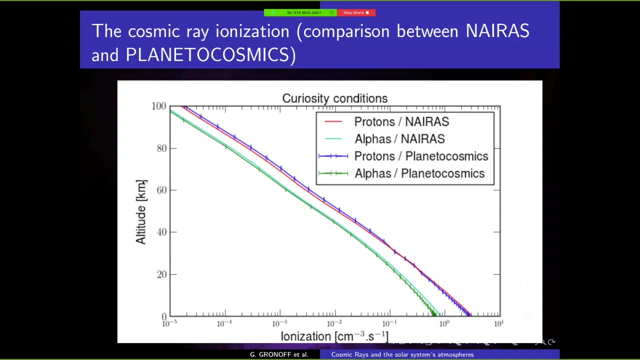 ionize at high altitude. But if you go back to the cosmic ray fluxes that we have here now, let's go and do the computation. What does it do? So we looked at NEAS and the planetary cosmic and we looked at the protons and the alpha. So basically the two. 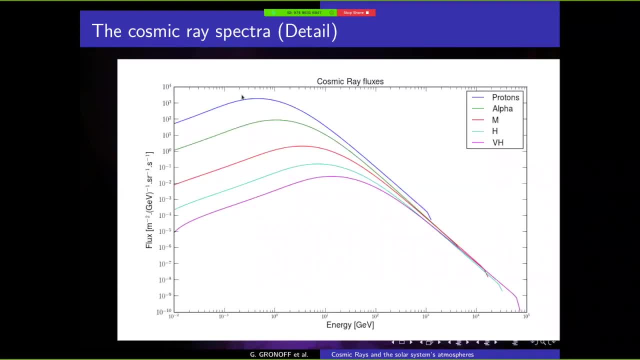 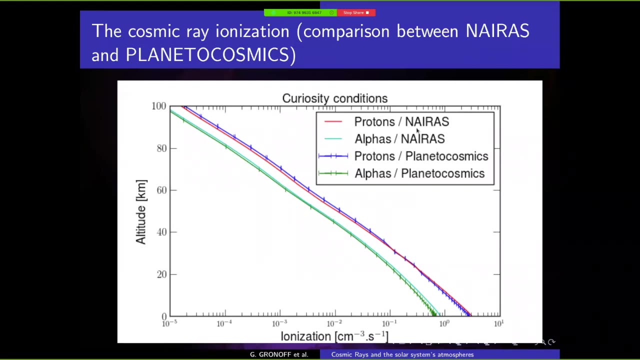 main particles going down there. I have some other calculation for this one, but it's not yet published, So in between we did the calculation at Mars for the landing of Curiosity, of the ionizing of the whole Earth. There's the Ionizing, Ionizing, Ionizing, Ionizing and the Ionizing, Ionizing, Ionizing. 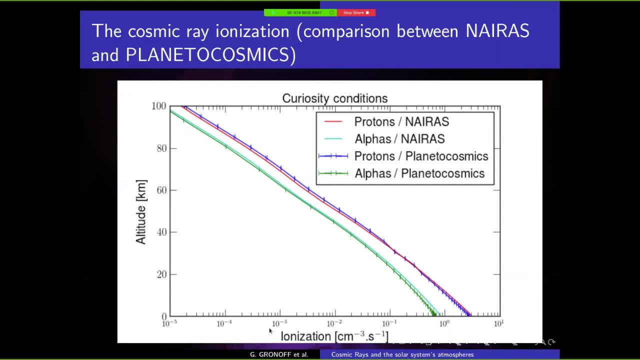 Ionizing, Ionizing, And we looked at the ionizing of the whole of the Planet And we looked at the rate at the ground for the different particles And we look at the difference between Planeto-Cosmic and NEAS. Planeto-Cosmic has small error bars here. 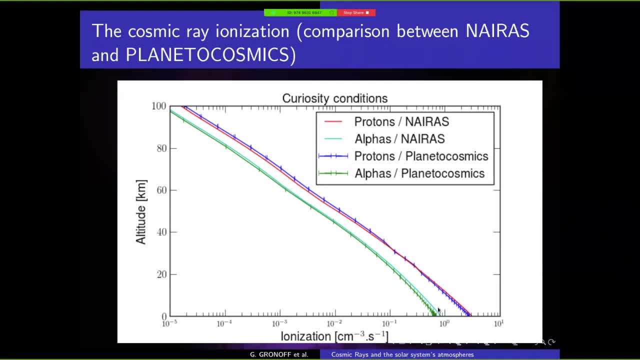 because it's a multi-carrier model. So we are able to do a little bit of statistics to be able to look at how the our calculations varies between each run, and that allows us to get a good estimation on the uncertainty that we have from the Monte Carlo calculation. 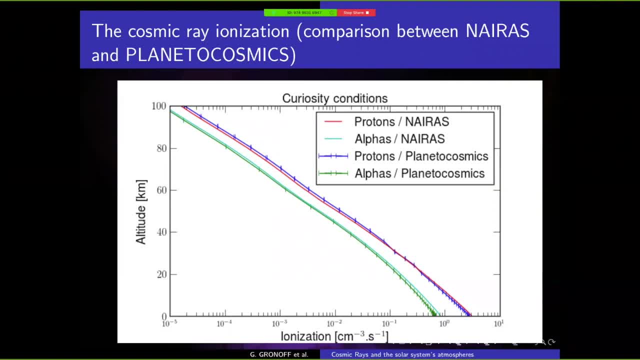 It doesn't. it's not a pure error, because if we have a bias, if we don't have real physics, that is not taken into account into that error bar. So overall we see that at the ground, at mass, we have two to three ionization per second, per cubic. 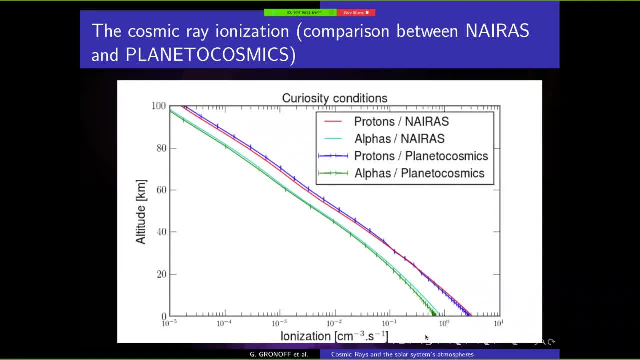 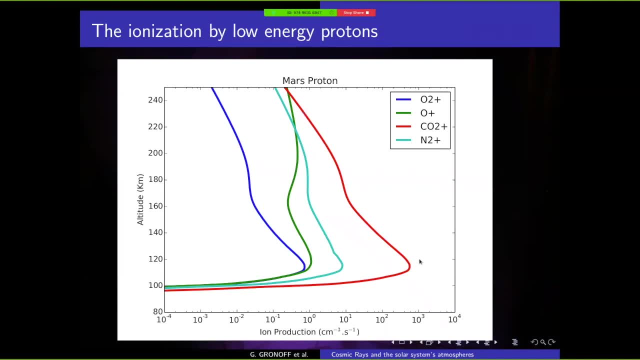 centimeter, which is quite a large quantity of ionization. When we look back at this proton ionization, you see that typically you have a peak and then you have you have the ionization going down. You don't have this at mass. 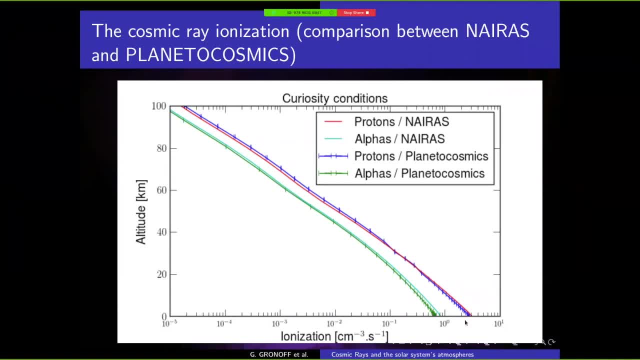 because there's not enough atmosphere at mass to see the peak for the cosmic ray. So there is way more cosmic rays that goes onto the ground And there is a part of this cosmic rays that go back toward the space, which is nice because we can try to do some physics. 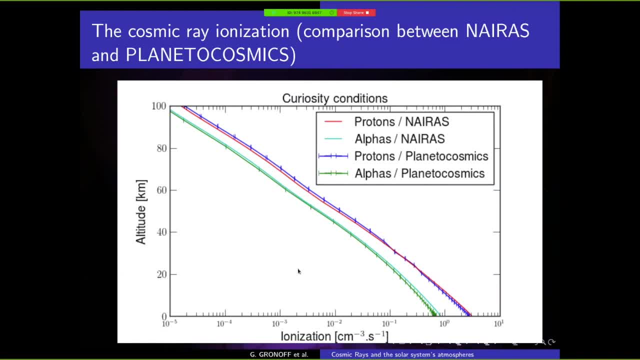 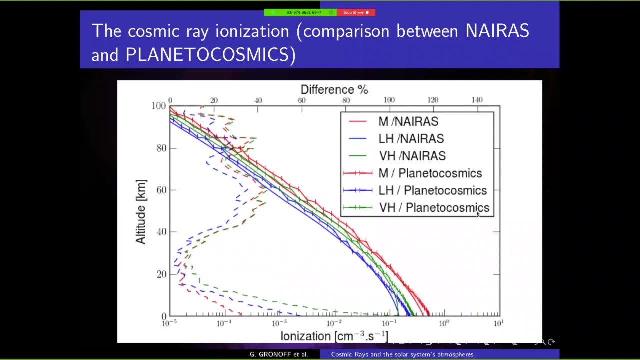 by looking at the cosmic ray that come back, We can do some physics that is linked to the ground but which is problematic for the astronauts, for future astronauts on the ground. Okay, so yeah, that's the higher energy ions, sorry, the higher mass ions. 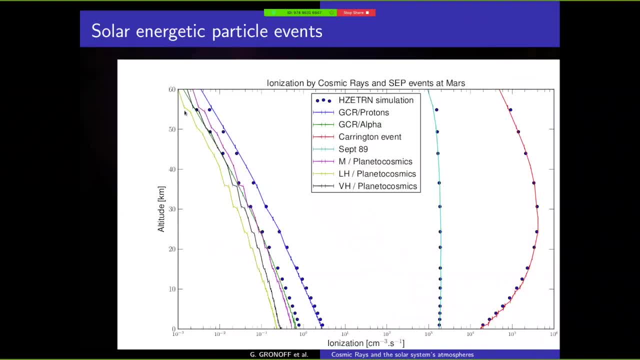 I will go through that quickly. So as an example, as an example of the problems that we can have due to the small atmosphere at mass, Let's look at the question of SCP events. So the SCP events that we have seen earlier that are very energetic. 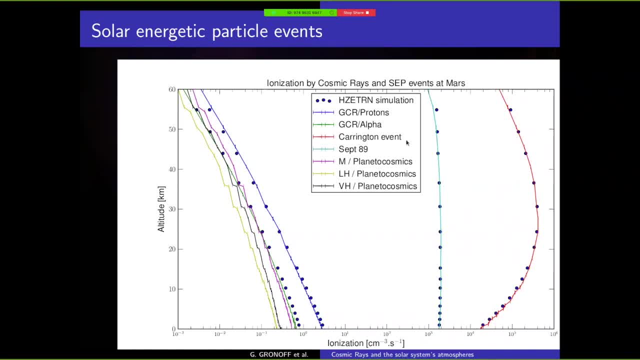 So it's a kind of an event. So that's an event in the 19th century that was totally crazy in terms of energy- Energy going out of from the sun and observed at Earth- And the September 89 event. So that was an event that was observed. 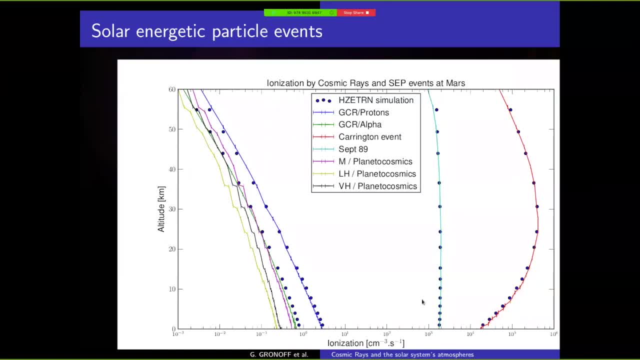 And what happened is that when we take this events and put them into the calculation, we see a large amount of ionization as a ground And, as you can see, it's a several orders of magnitude More so counting one about it. so that will constrain what cost friction of the spectra. 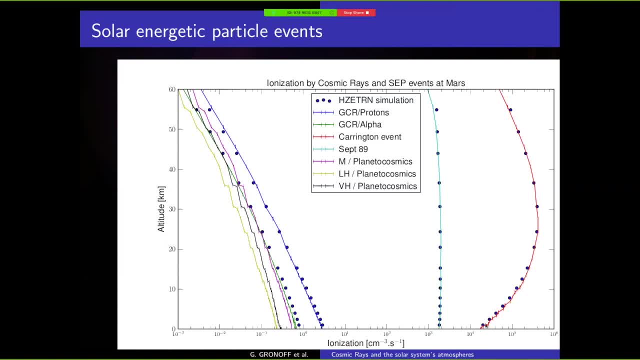 So we it's just something for, but for this event it's way more solid in terms of ionization. This can be big And since it's big, it can be dangerous for anybody going over there. So we have to address: how much does us? 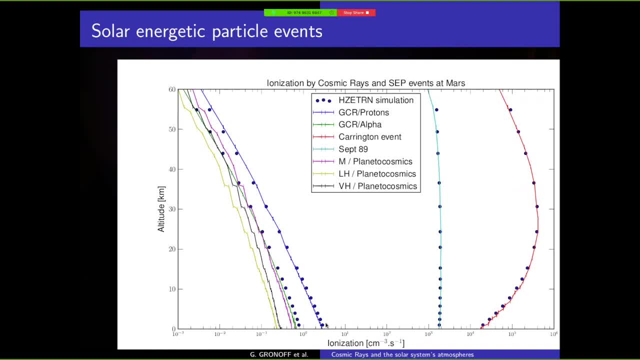 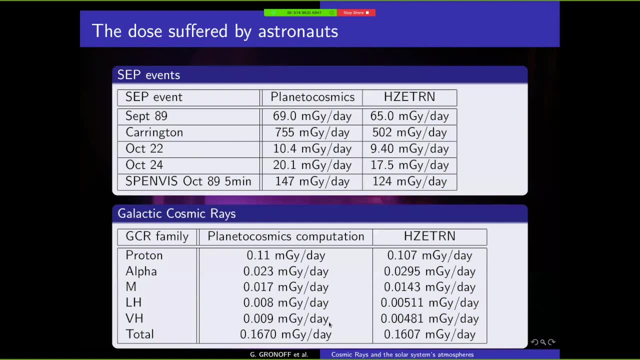 it gives to astronauts. So now let's go to dose. So dose is in. so it's really the amount of radiation that is absorbed by the body, and what happens is that we typically put at 20 mSv the dose that somebody should not go above in a year. 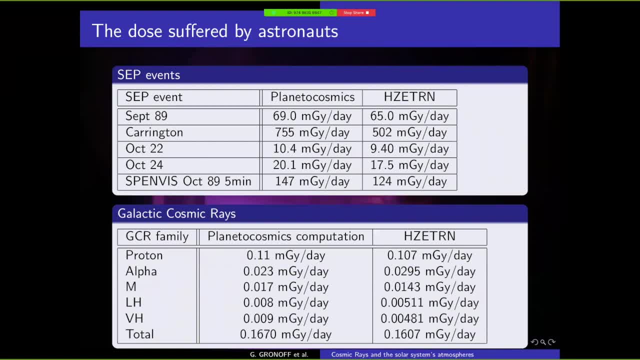 as a civilian. So a mSv is a very difficult unit because it's not only the dose in a kilogram of matter, but it's also it has a weight in function of where it is going It's and from which kind of particle it's coming. So, for example, if you have 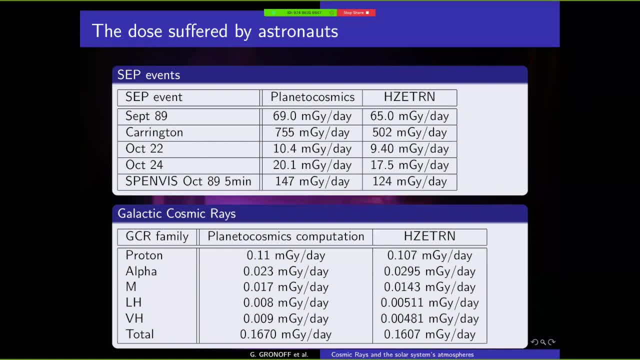 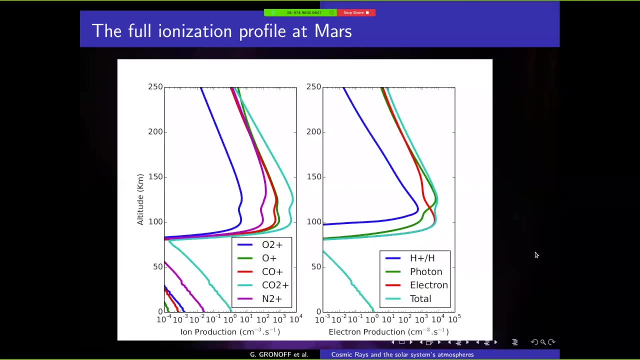 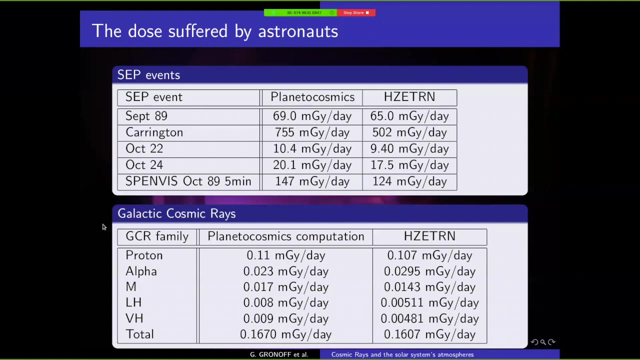 a gamma ray. the gamma ray will go through your body. it will deposit some dose, but it will not. it will be less likely to make huge damages to the DNA, for it will hear me, Yeah, Okay. So going back to all this, this events, so, mSv, it's complicated to. 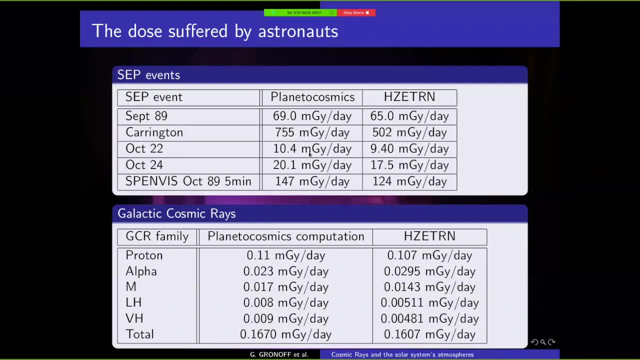 compute, but mG it's more easier to compute. So, going there, we, we took a, we took our code and we computed the dose in mG in the ground And we have to consider that it is a little bias between mG and mSv, but a rule of thumb, you don't want to be. 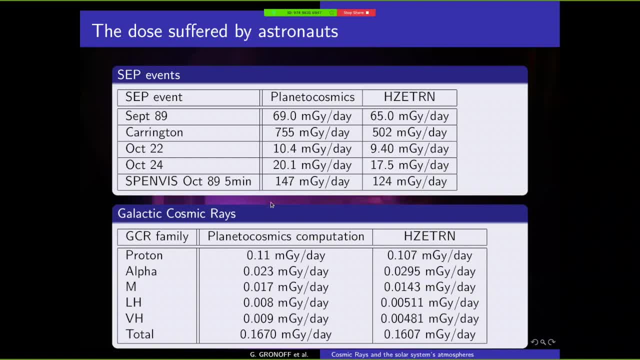 above a hundred mG That's. that's really bad in the duration of a mission. So you want to have just just a few fewer irradiations than that. And when you look at the SCP event computed by both system, you see that we can if we have September 89th. 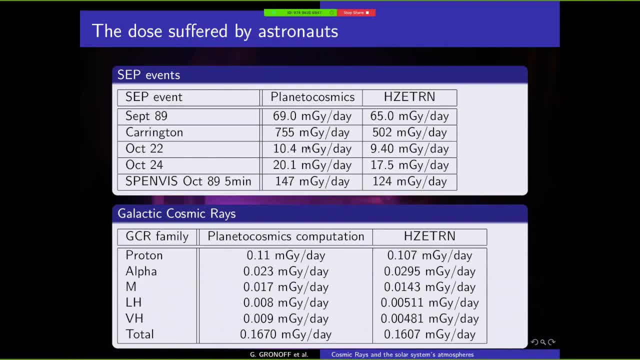 or Carrington event, we start to have huge amount of radiation coming in a day, So this is where you have to protect your astronauts from going out so that they don't get affected. It may just be one of these small tailings that they are completely found. 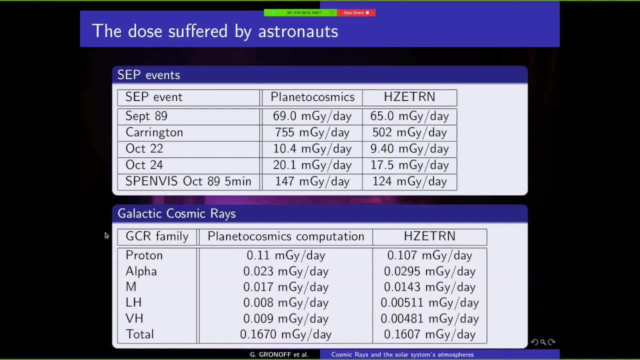 inner At the curry off. When you look at GCR, it's uh, it's a little bit better, but you still have to be careful to not but you astronauts too much out in in in the field, because in a hundred days you go. 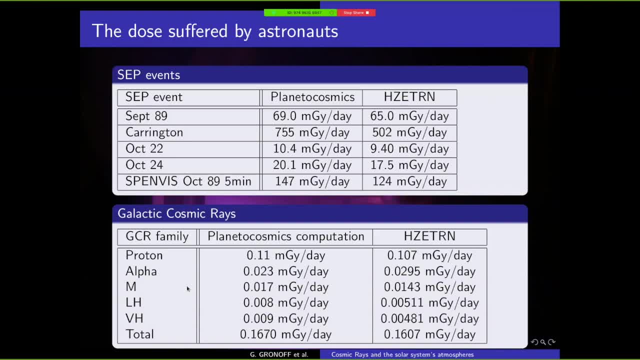 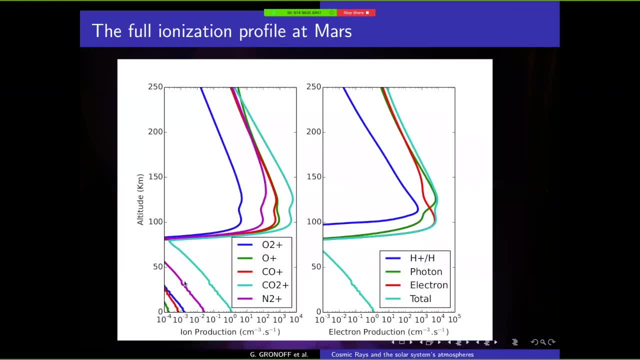 and you can even adjust the astrology. as I told in Jавard's presentation, I used to calculate a hundred days and you can easily go above what is the baseline for everybody. This is a full ionization profile at Mars. I'm going to go a little bit quickly here, but 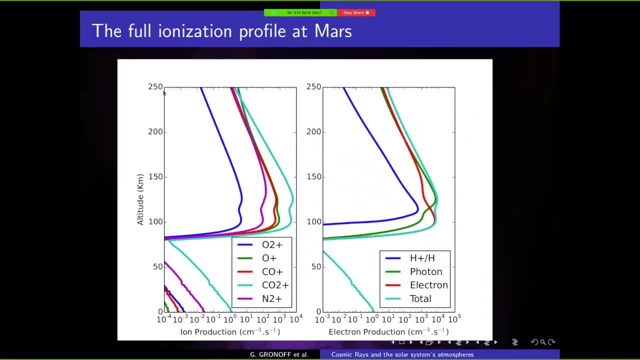 this is what we do when we do computations of everything, And this shows a little bit. what is the big comparison between what we have in the top of the atmosphere and at the bottom, still showing that the top of the atmosphere really prevents most of this ionizing radiation. 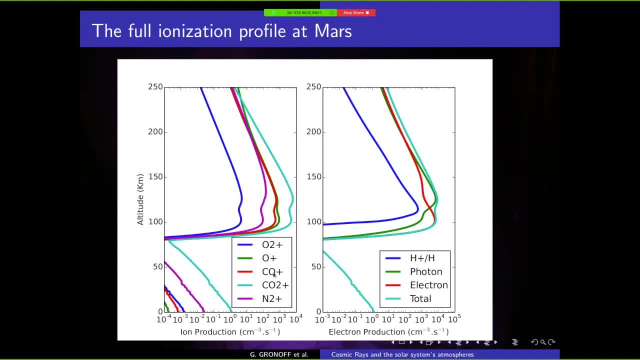 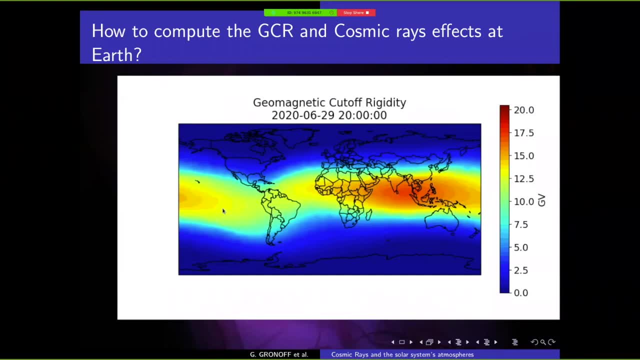 to go down, even if those are less energetic and more easier to shield from. And now let's go, since we are speaking about shielding, to the Earth. The Earth has a big difference with Mars. it's a big magnetic field. A magnetic field has an effect on the particle, on the GCR. it's preventing them to go down to. 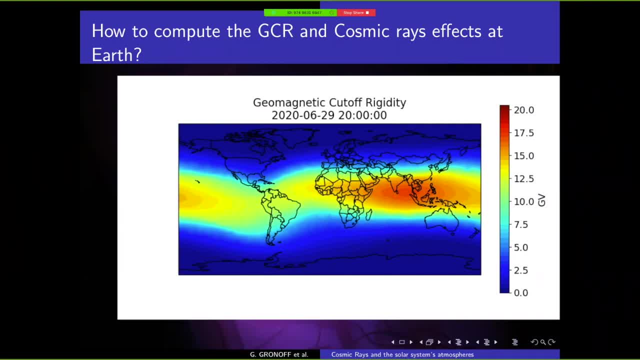 the atmosphere. It can make some of this GCR go back to space. It doesn't work everywhere. because you are near the pole, all the gcr can go down in the atmosphere. But when you are in a low latitude to mid-latitude you can be effectively shielded against the less. 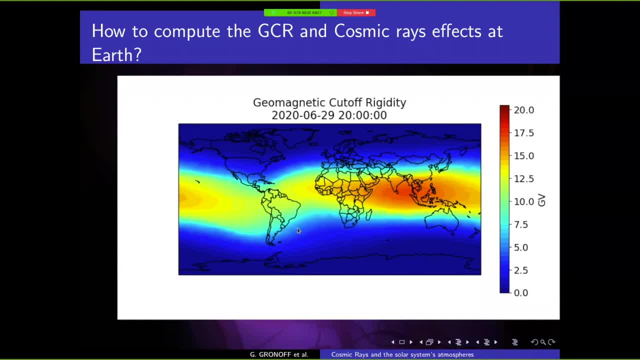 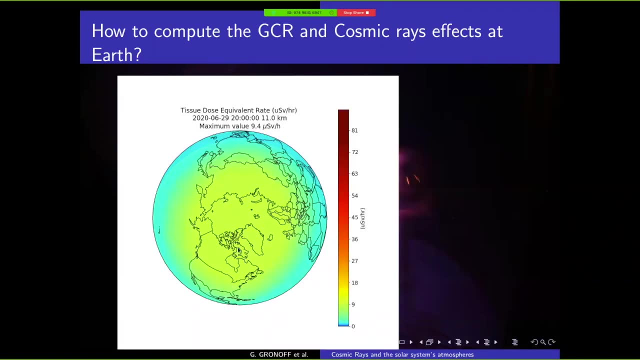 energetic particle. So if you start to go and fly at different altitudes it will affect the amount of particles you receive. So here I did a calculation from yesterday on this ionizing radiation and how much microsievert power you have in those equivalent from a flight. 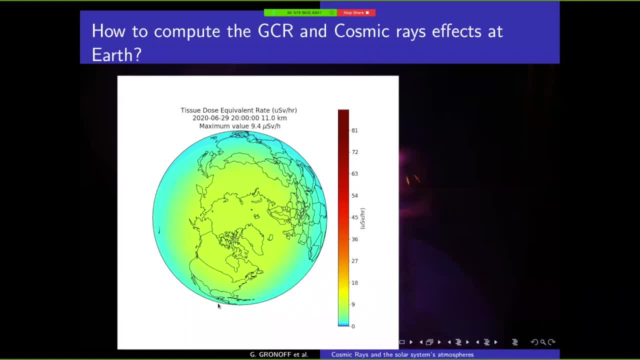 So it was not a lot of ionization. We are in green, green-orange at 11 kilometer. If we are going a little bit higher it's a little bit more yellow And of course, if we were to fly with one of these new small rockets and go very high, we would have a big 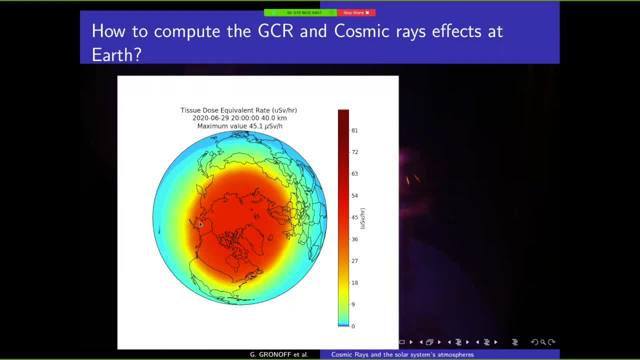 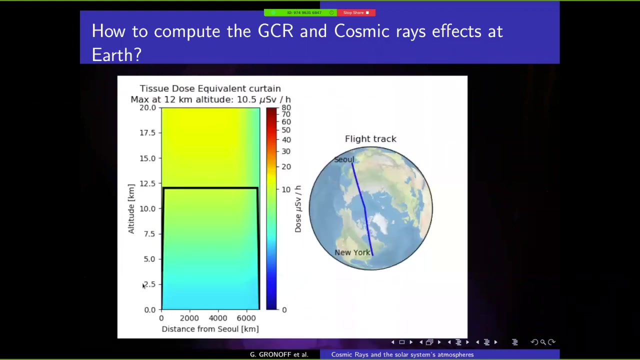 dose if we flew at this high latitude, And that's a big advantage of NEAS: It's able to compute all of these problems and give us an idea of what will be the dose from flight to more complex vehicle like this T Montreal customization. 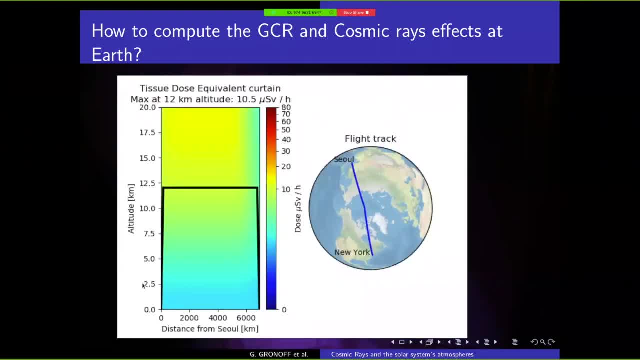 rendering THE is to be able to compute, if we have a flight, to see where it goes, how much time goes, at which attitude. compute, the dose that the crew will suffer each time. And that allows us to give an idea to the crew. 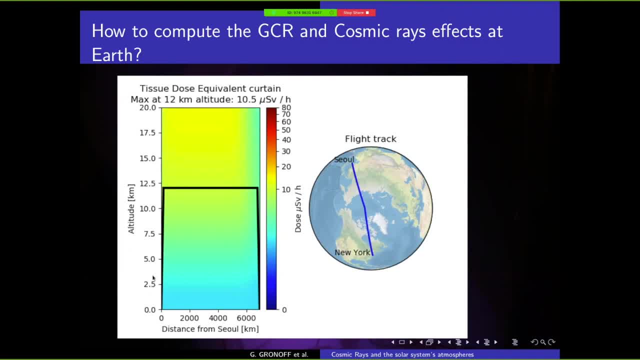 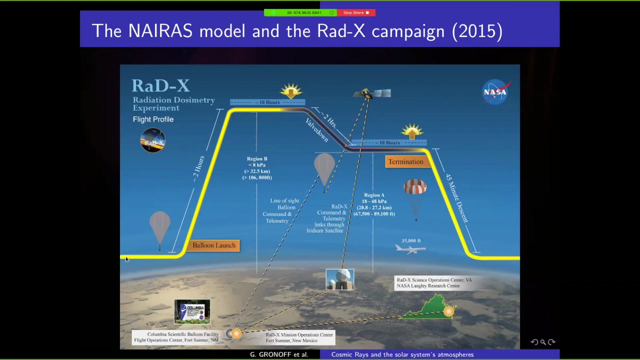 of how much dose they suffered during their flight and during their year, to see if they are able to go above their level or not, And it's important, especially for pregnant women, to have a good idea of what's going on over there As a way to validate our codes. 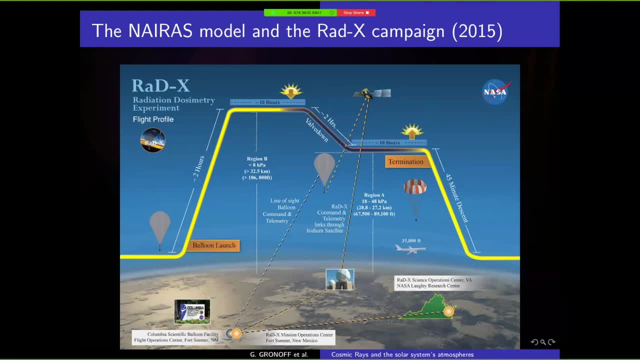 and to look back at all of these problems we had. we have a lot of campaigns, measurements And in 2015, we did that HADx campaign to be able to see how it goes And to be able to validate the model at high altitude. 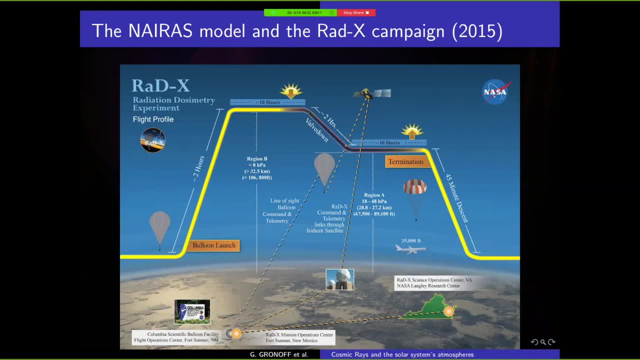 because it's one of the main problem. So I was able to participate in that mission and we had a very frank for 10 hours to get most of the radiation from, just from the cosmic rays, So at high altitude to see what is coming down. 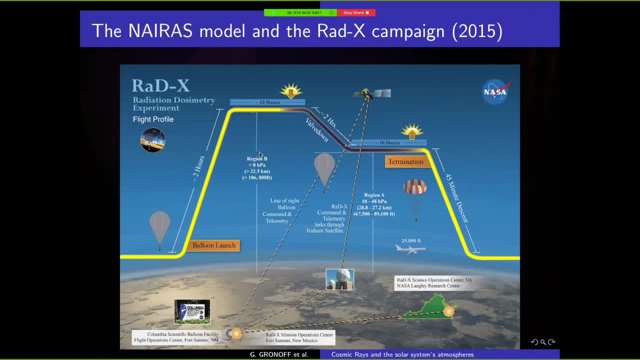 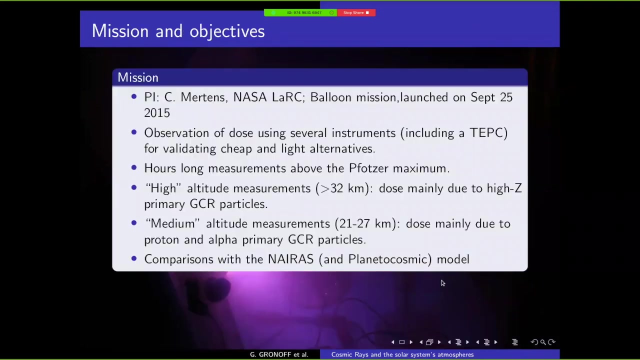 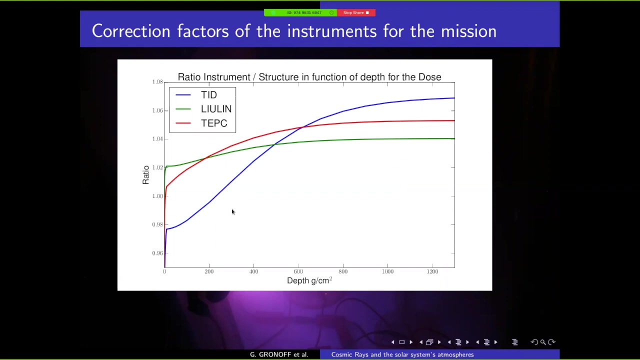 from the high Z, so the high mass cosmic ray, And then we go at low altitude to see what is coming down. It was quite a complex mission and my work there was to do some work on shielding of instruments. That's something that we can do with the cosmic ray. 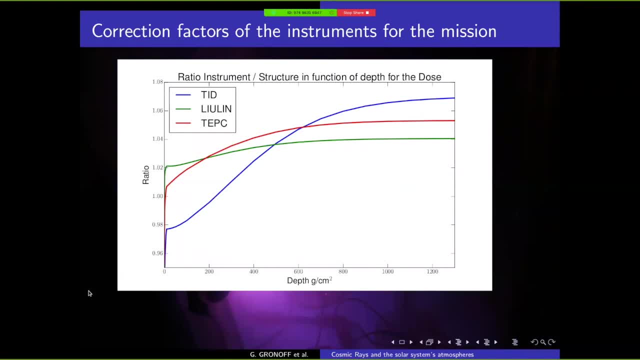 So there's a petrocosmic model and the giant force to see how the shielding of an instrument will affect the dose of radiation, to see how the shielding of an instrument will affect the dose of radiation And how the field pixels looked by the instruments. 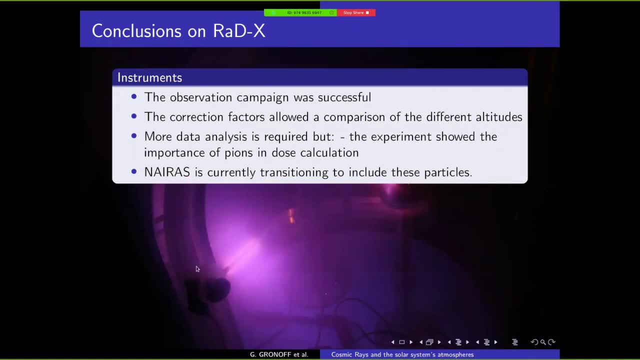 And so it was nice for this kind of validation. And so it was nice for this kind of validation- and it's still something that we are analyzing right now- to correctly improve the NERES Standard and have better estimation of those for the crew and because different flight and how the aircraft 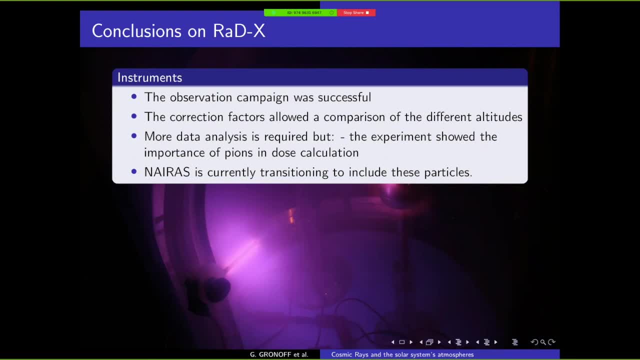 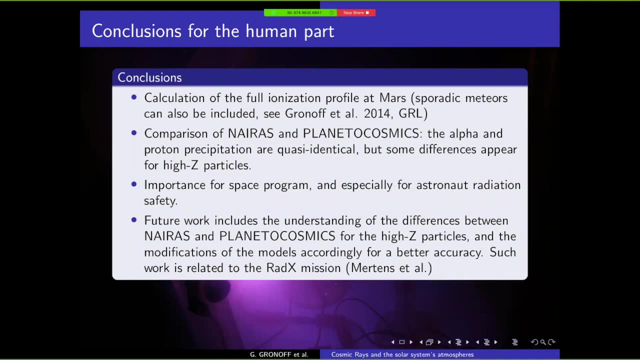 that will also affect our work on Mars, for example. So conclusion for that three part of human exploration: it's important for a space program to be able to look at radiation and radiation safety And it's really good to be able to go into the details. 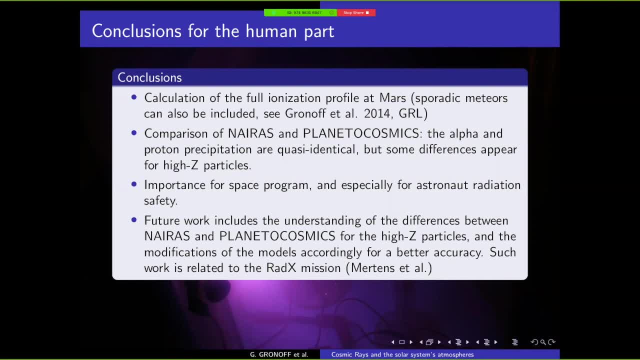 on all the sources and where they affect the crew or they affect the instruments, And that allows first to understand what we are seeing in the atmosphere and then to be sure that the people who are in the atmosphere, the people, are safe while going in space. 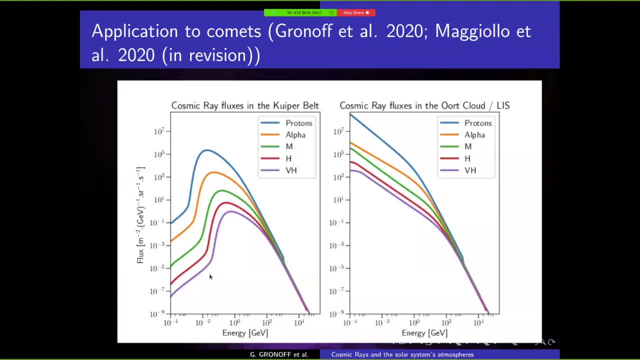 So how much time do I have? You have about five minutes, Okay. so yeah, I'm going to go very quick on this part. I'm going to show you a couple of the latest results. So very quickly. First, we were speaking earlier about the effect. 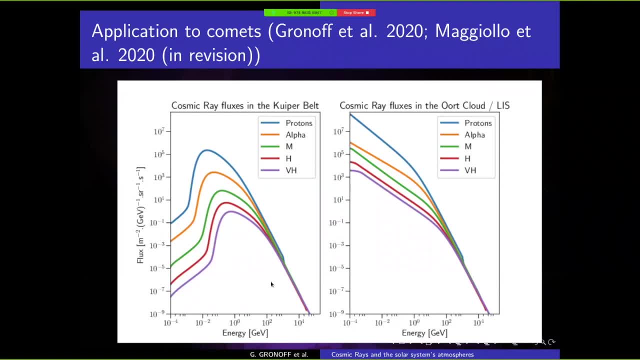 of the haos here on the cosmic reflexes. Here we are going into this big effects. So you see the energy in GV here and here we are out of the solar system And it's what we think the cosmic reflex look like out of the haos here. the local interstellar spectrum. 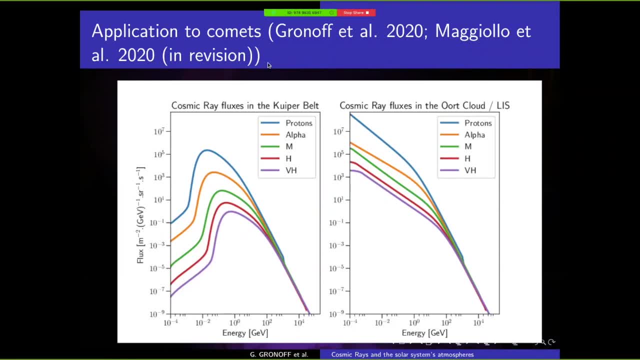 or the earth cloud, And here it's what we model in the creeper belt. So you see that the effect of the haos here is quite dramatic on the amount of cosmic ray around the hundredth of MEV to a GV And one of the objects that it's really impacting. 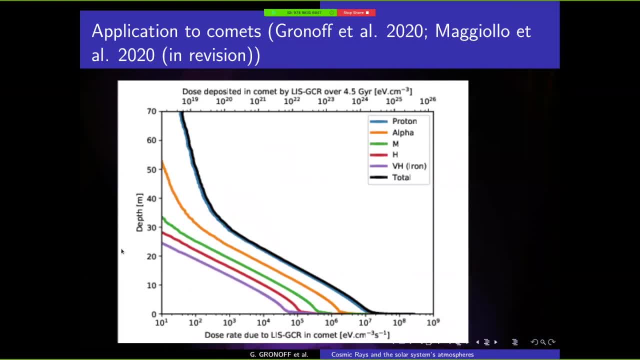 it's comets. So in a couple of paper that we have been working, the first one is published and the second one is being reviewed. We have been looking at those deposited in comets. So either per cubic centimeter, per second. 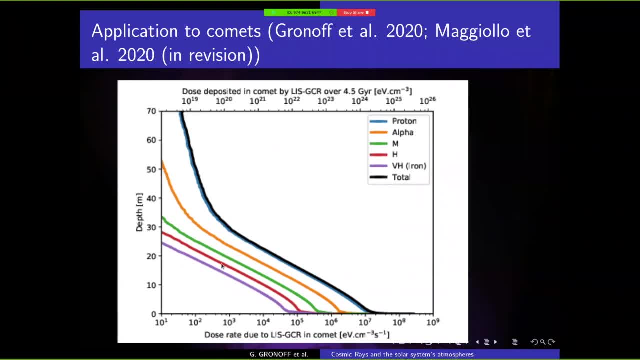 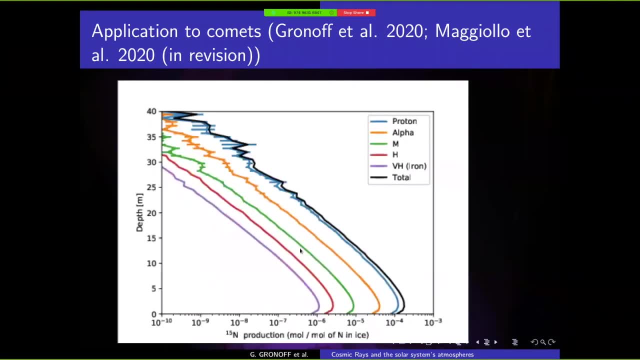 or over the last 4.5 giga year, And we looked at the total amount and it's quite important. It's really interesting because it has an effect on the isotopic ratio And it's very close to the levels that are needed. 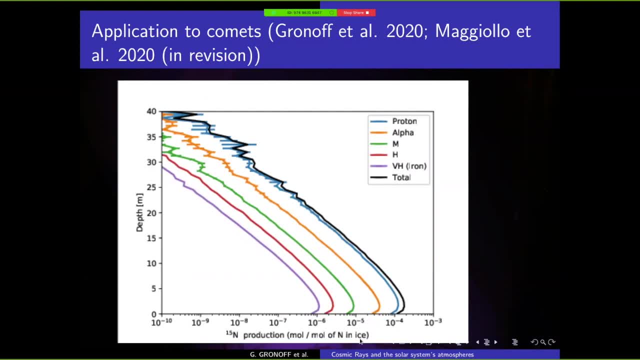 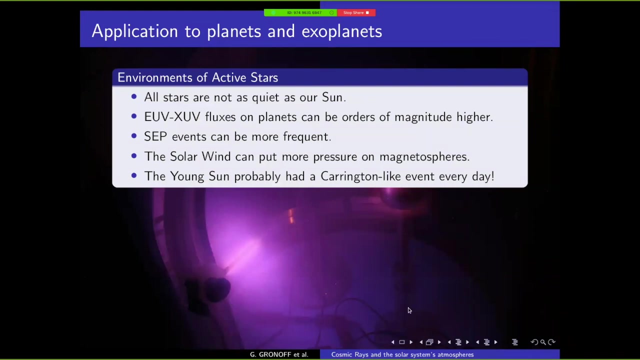 to change from a ratio of N15, that is, a stellar- to a ratio. that is something that we are observing right now. So that's the first thing, the first of the effect. Then we have an application to exoplanets and the early earth. 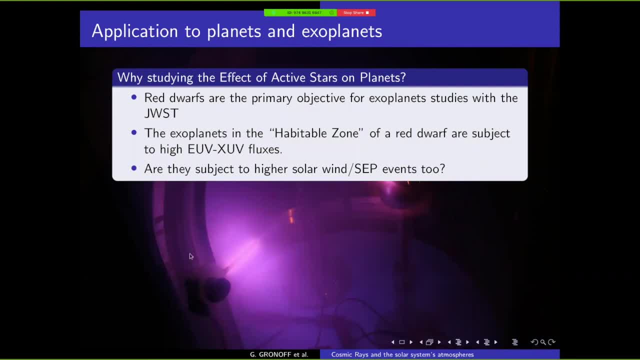 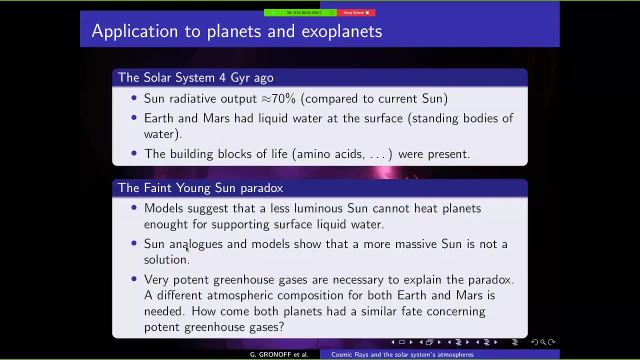 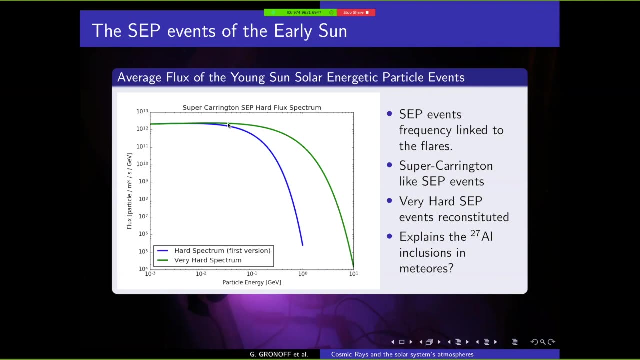 And I'm going extremely fast here. It's it's based on the 2016 paper. by So going very fast, The idea is that we had very high HCP fluxes in the past in 4.5, sorry. 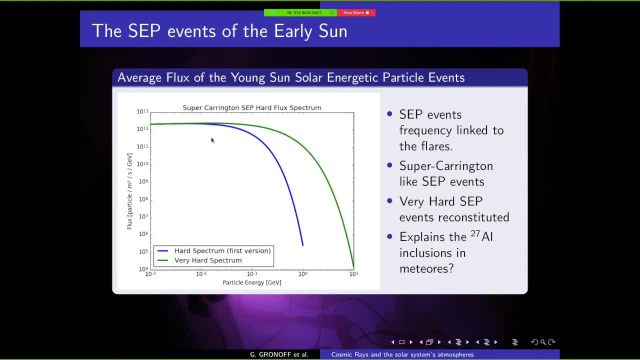 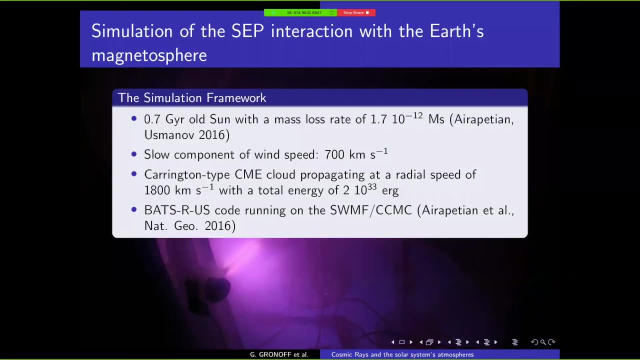 four giga years ago, And it was at the time that the sun was fainter and was not really able to hit the earth to have liquid water At the surface. but we had liquid water at the surface. So what we have been doing is that we have been looking. 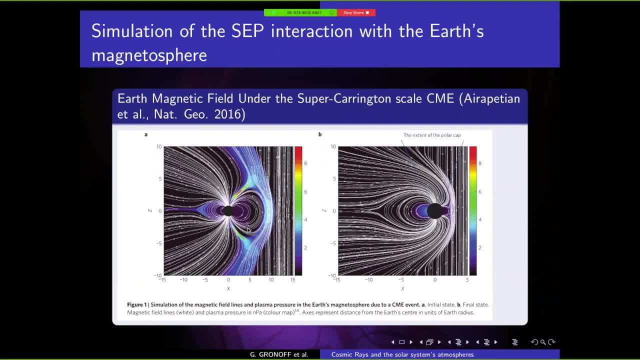 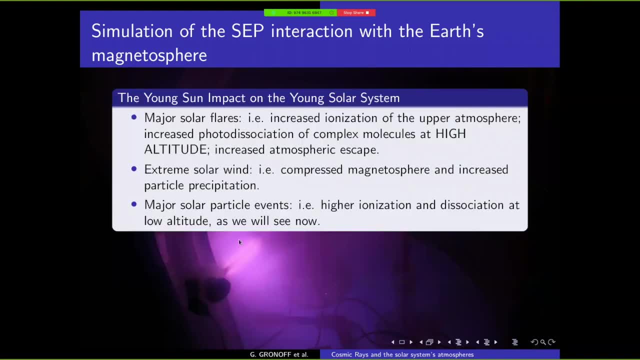 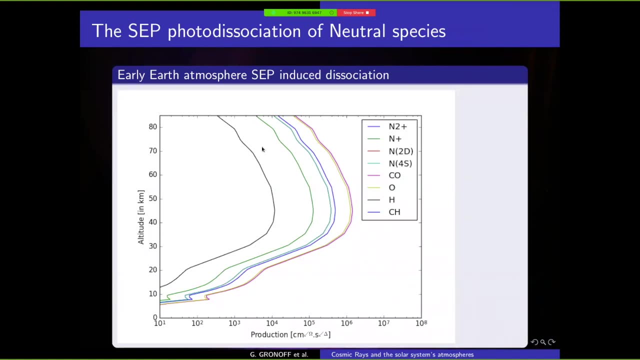 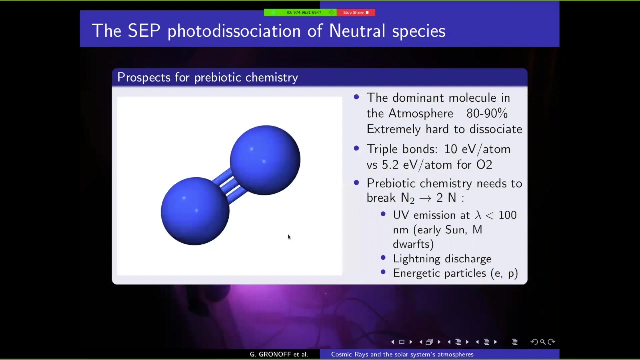 at this very big stellar solar events, looking at how it compresses the metasphere and goes inside the earth. We computed the creation of radicals and ions from the solar energetic particles And especially, and we looked at the creation of greenhouse gases from. 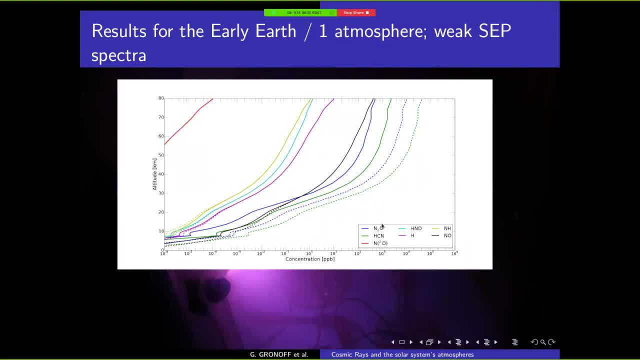 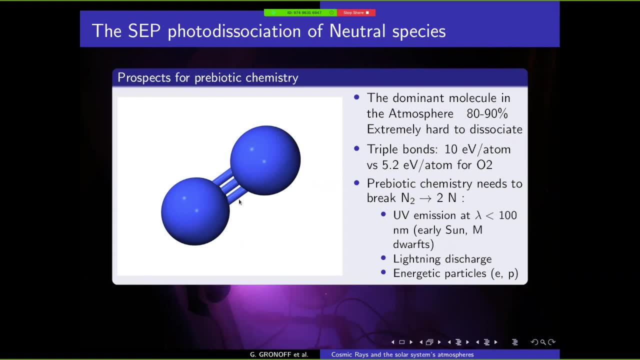 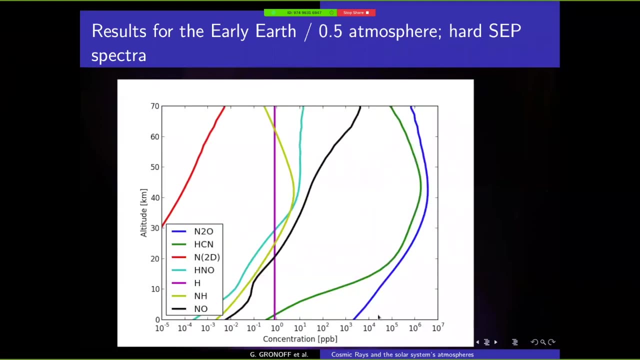 from the and especially N2, which is very difficult to create with with other processes, because you need to break the triple bond of nitrogen And we go to have a concentration of nitrous oxide. nitrous oxide start to be quite high. 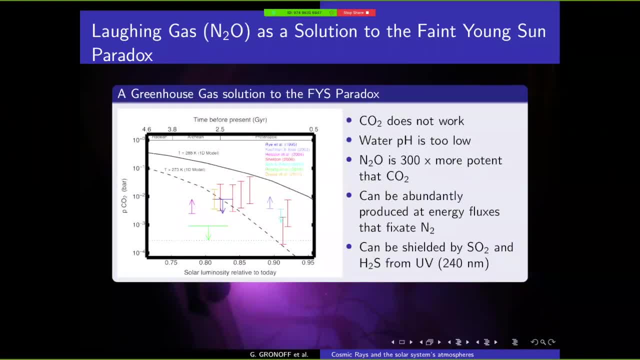 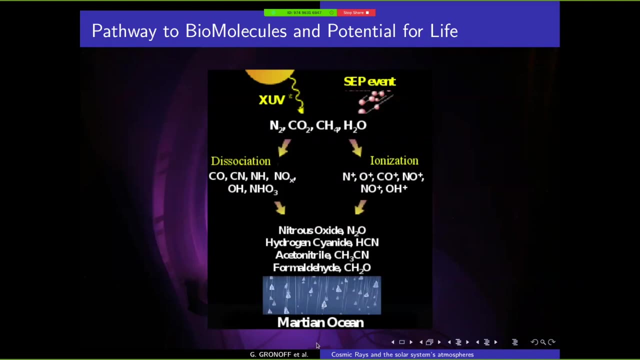 And that can really help in solving the Fent-Yongson Paradox by heating up the atmosphere of the young earth. In addition, there is something very interesting. with all these sub-processors It's created nitrous oxide, hydrogen cyanide. 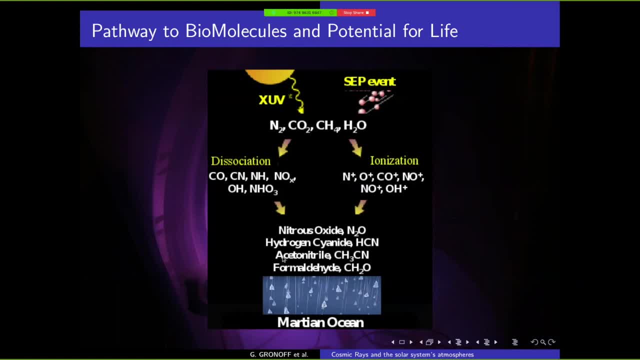 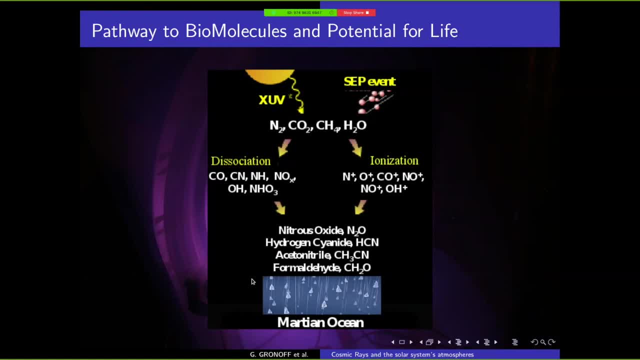 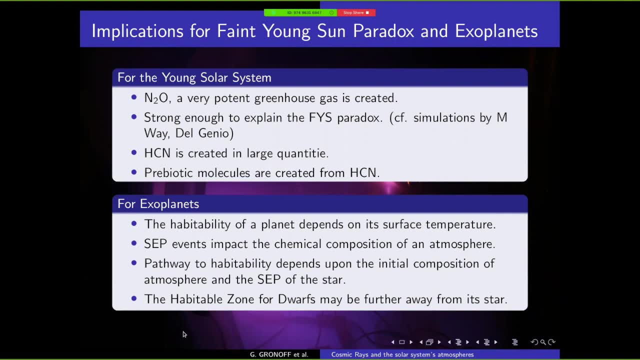 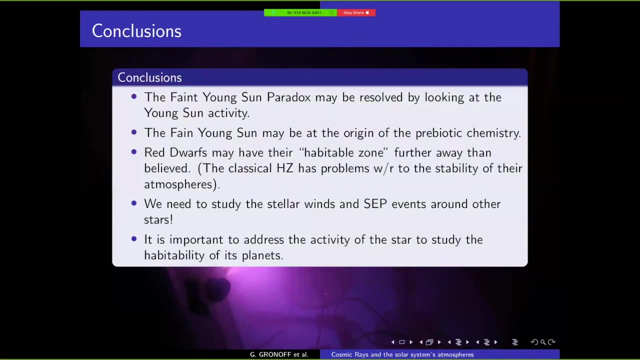 in the remnants of the Martian ocean. So it's, it has big implications for the field of astrobiology, for understanding our past And- and that's a question- that's something that is very interesting to look at. So yeah, it's, we have seen that the cosmic ray 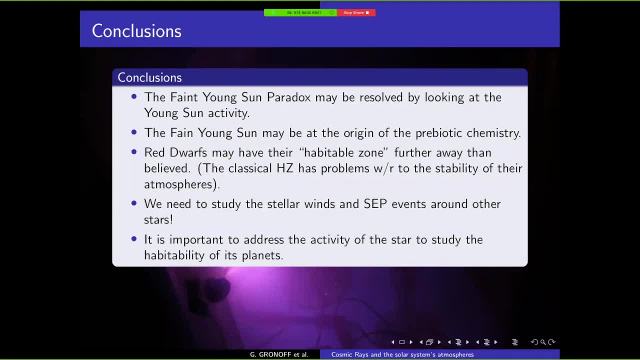 are very interesting to, are very important to address for space exploration, human space exploration and for everything for instrumentation that goes over there. I've shown you very quickly that it has impact on the weathering of small bodies And that weathering is something that is important. 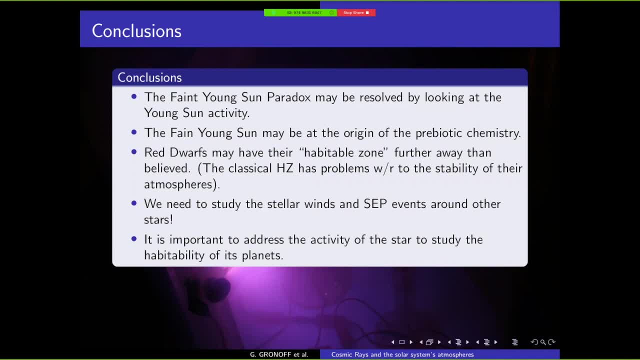 to understand if we want to look at the history of our solar system from the observation of the small bodies. And finally, I've shown you a couple of impact of the SCP event and the cosmic rays on the atmosphere of planets And on the effect of evolution and creation. 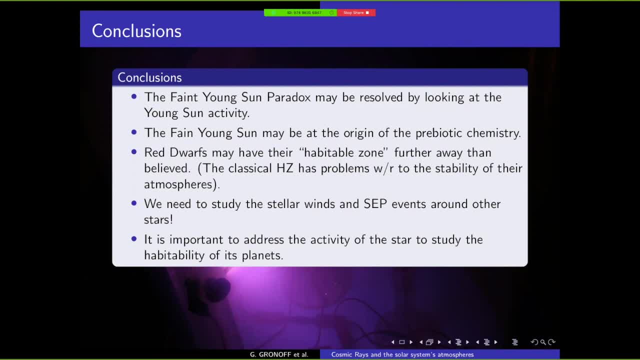 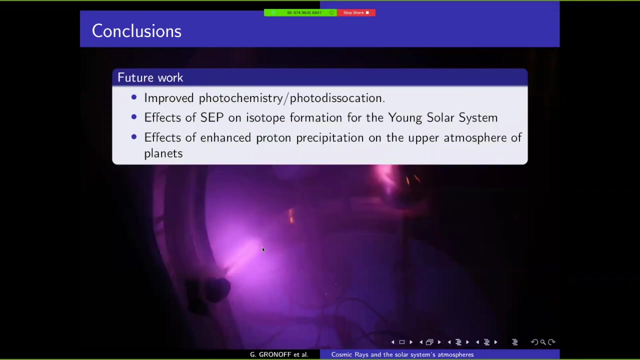 of important molecule for the origin of life and for everything that is of interest to understand how an atmosphere evolve and maybe to understand why our Earth was not totally frozen in the past. So there's a lot of work to be done from there. We have way more work to do on that latest hypothesis. 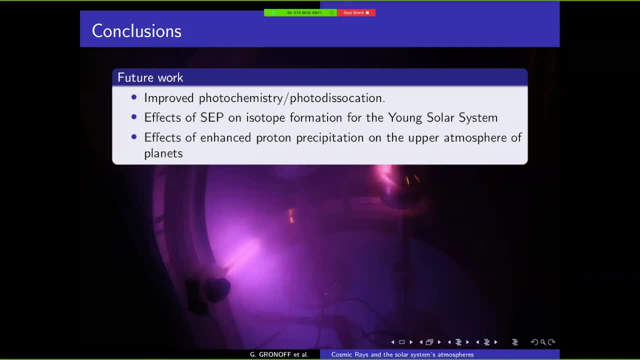 to improve our chemical model. We have more work to understand the SCP and to better address the effect even on the human space exploration. And we have much more work to do to better understand how that affects the upper atmosphere of planet, especially with the crime of escaping processes. 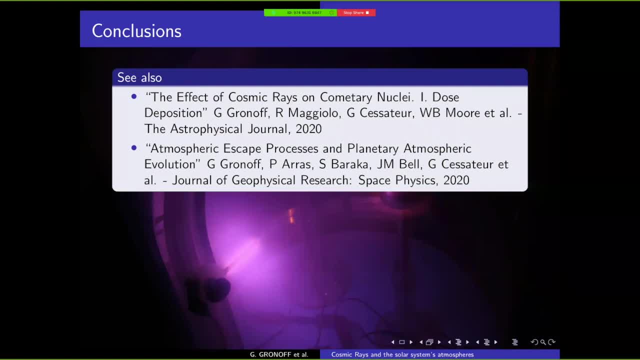 on the atmospheric evolution. So I am putting here a couple of papers that have been recently published and that show a couple of the future approach that we are taking here. And well, I will thank you for your attention And I still I want to apologize for this little block. 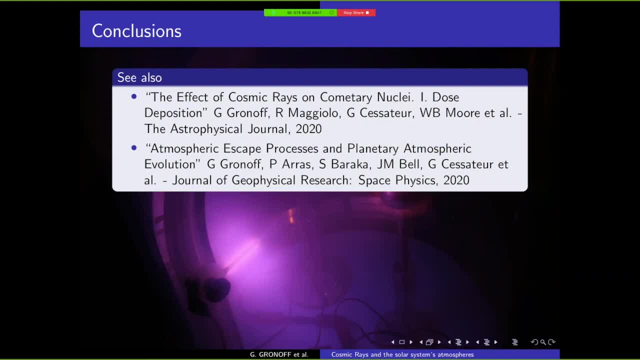 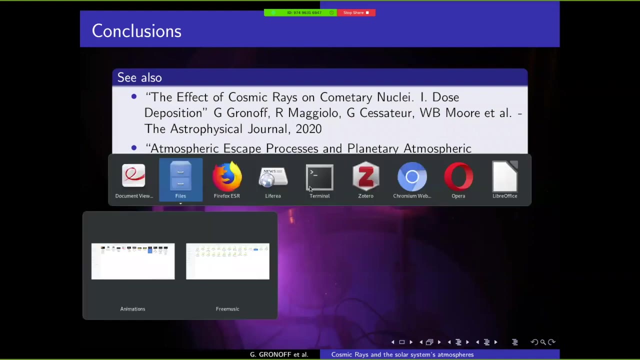 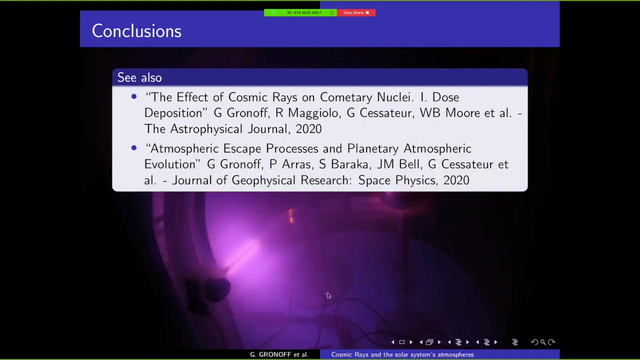 in my internet here. Okay, that's all for me. Thank you All right. Thanks a lot, Gun. Okay, Yeah, So let us start with Q&A. Yes, Srini, you can simply ask him. Your mic should be working. 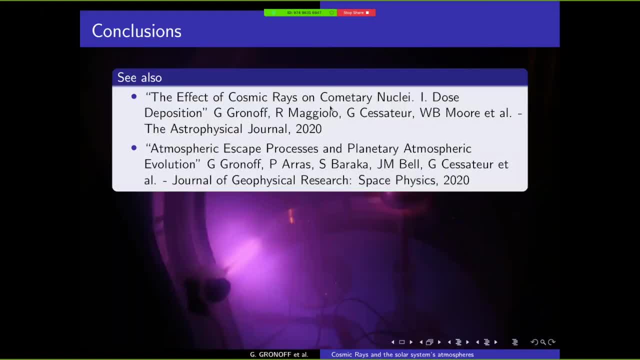 I just asked you the question: Can you somehow quantify the effect of all this on communications? Ooh, that's a big, big question. So there is a communication at. are we speaking about the Earth's communication When we start to going from? 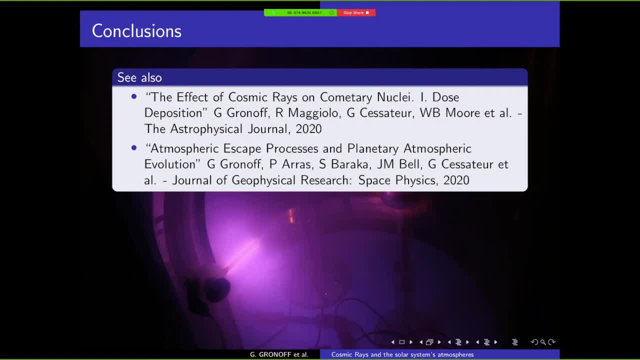 From satellite. Yeah, satellite communication, So it has. so there is two big effects of cosmic ray and STP on the on communication. The first effect is really disturbances in the ionosphere And that will so when we ionosphere. 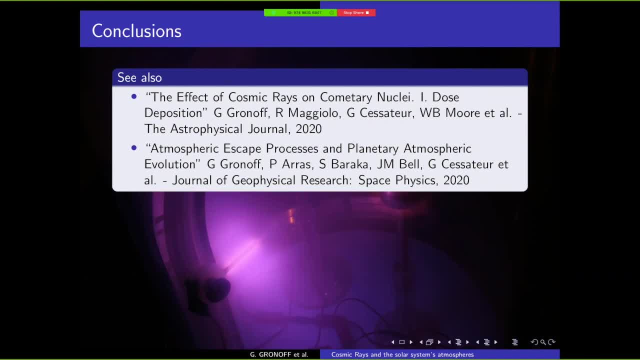 that will so when we ionosphere. that will so when we ionosphere. that will ionosphere. that will so when we ionosphere. that will so when we ionosphere. that will so when we Ezionize more. 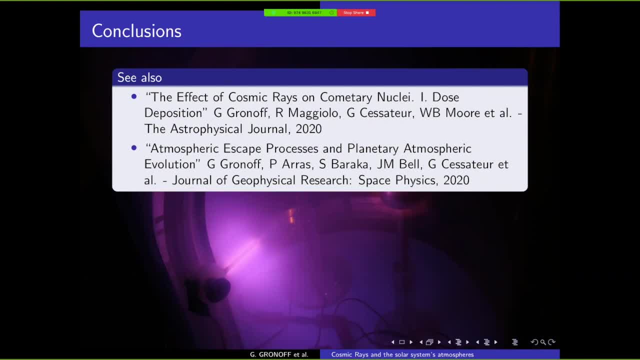 we start to create more, a different plasma, So the plasma is different, so the plasma frequency is different And that can cut to communication between the ground and the and the satellites. Usually it's not a big problem because we are far from the cutting frequencies. 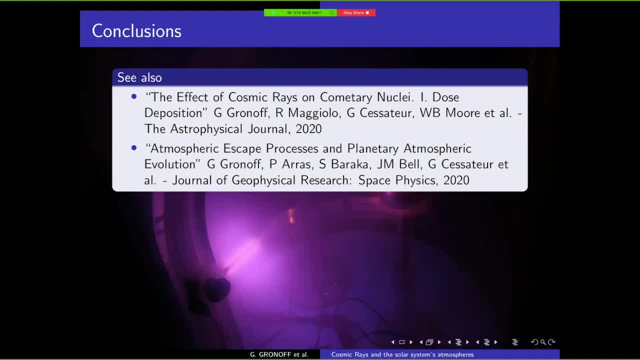 but that's something that is of course addressed in the tryna And, yes, in the code that look at this communication problem. On the other hand, if we start to put more ions, we can bounce a little bit more easily some radio signal and so the radio amateur radio. 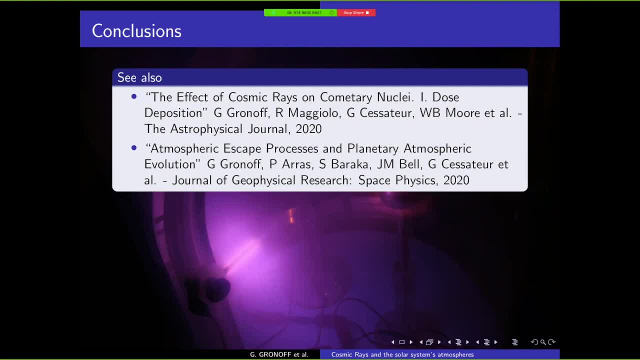 like to have stellar activity, solar activity that is higher, because they can communicate more. And, of course, a big point of this study is also to prevent having communication losses with planes that are going to high latitudes, because that most created a lot of problems in the past. 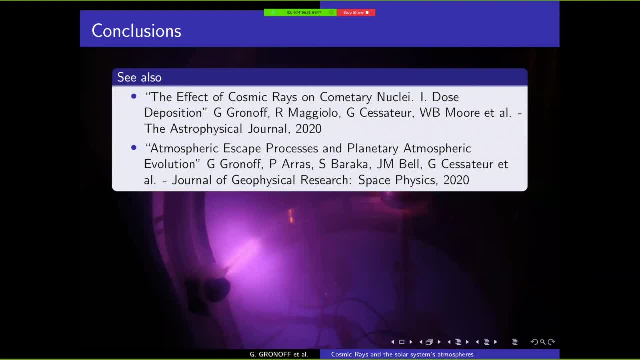 So that's really the first and the biggest concern with this: communication losses. Then there is, of course, having a huge storm that starts to knock out satellites. That will be a big problem And that's why it's important to be able to put satellites. 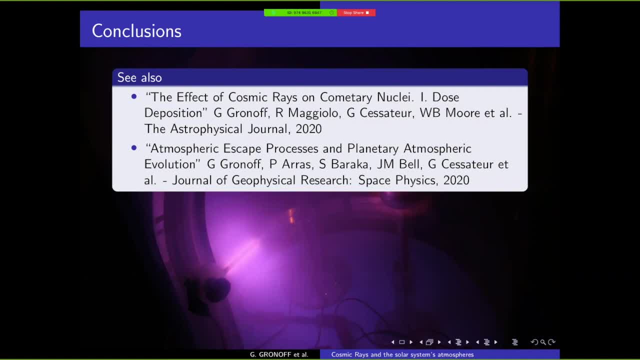 in safe mode before big storms So we don't lose these different satellites. And that's really the idea behind the space weather is to try to address all these effects And we don't want them to be bad for the operations. All right, thanks. 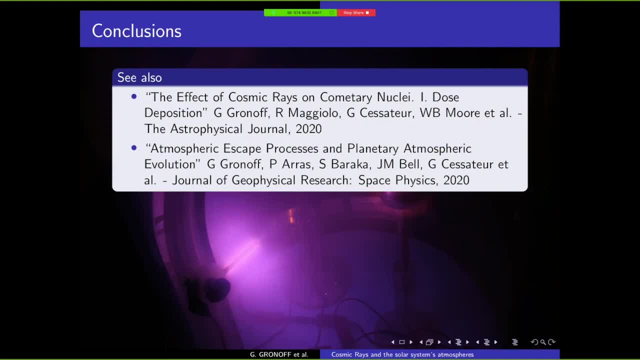 Yes, so we have another question, Reza, please go ahead and ask your question. So thank you for your presentation And yeah, so my question was about the ionization accuracies and you mentioned that the NIRAS and planetococosmics. 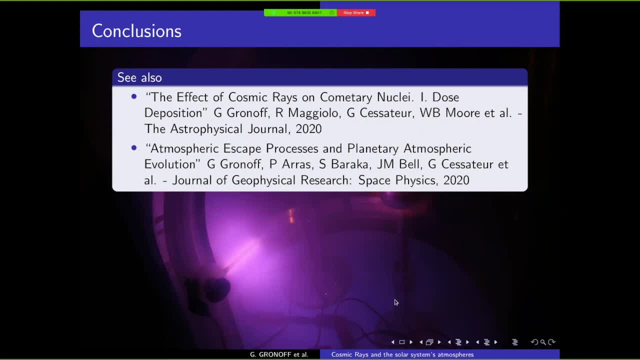 they varied in the space weather. They varied in their efficiency and accuracy. So one of them was very accurate but took a lot of time- computational power. but the other one was less accurate and performed computations faster, But in the cosmic ionization slide. 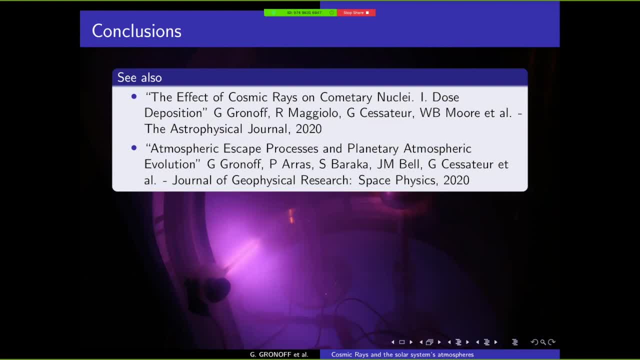 you showed us where the ionization values were against the altitude, that their accuracy for a particular altitude were pretty similar. So in what ways do they exactly vary in their performance? That's what I wanted to ask. Okay, so let me go to the one slide. 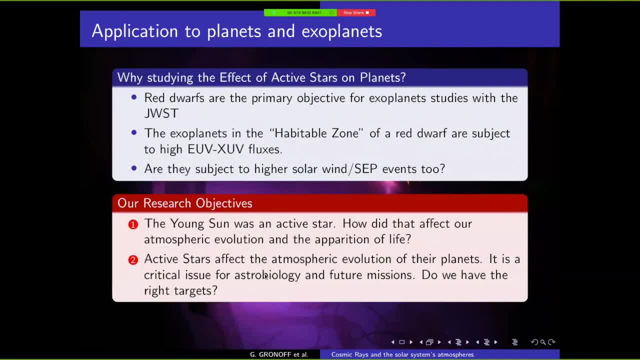 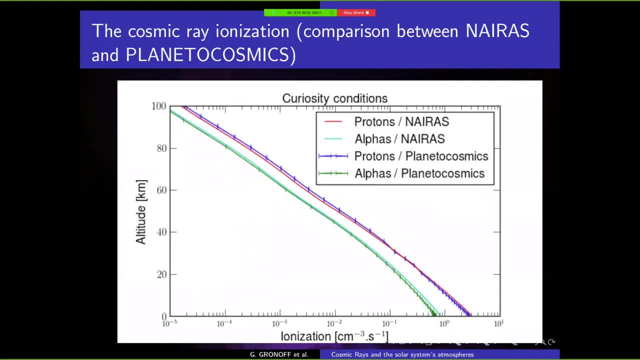 Okay, so let me go to the one slide. Okay, so let me go to the one slide That I went through very, very, very quickly. That's a high. So what I did show you where it's nice it's when you start to get with protons and alpha. 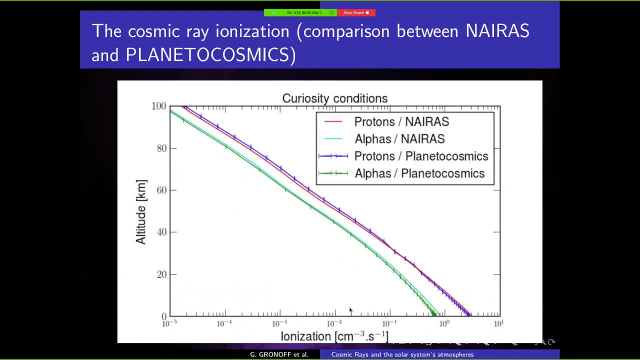 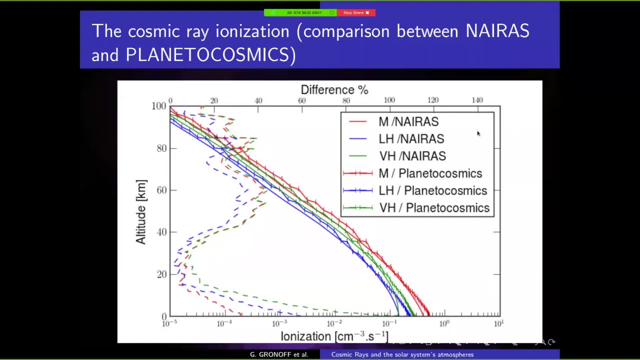 And you see that it's 10% difference, five to 10% difference. But when you start going to the higher mass cosmic rays, then you see to, you start to see, you start to see difference in the 30 to 40%. 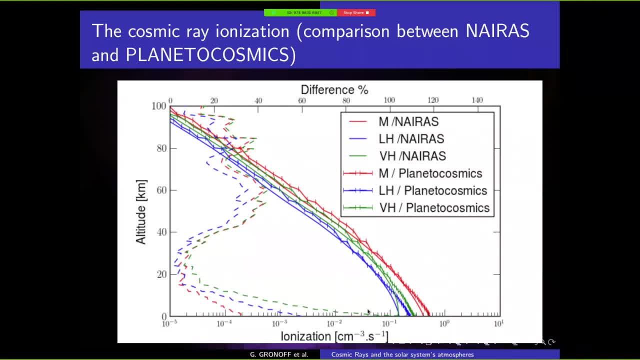 And you can go to very high percentage difference. So this little you can see my pointer here. So this little you can see my pointer here, I'm sorry. Yeah, so this line here, it corresponds to the difference in percent. 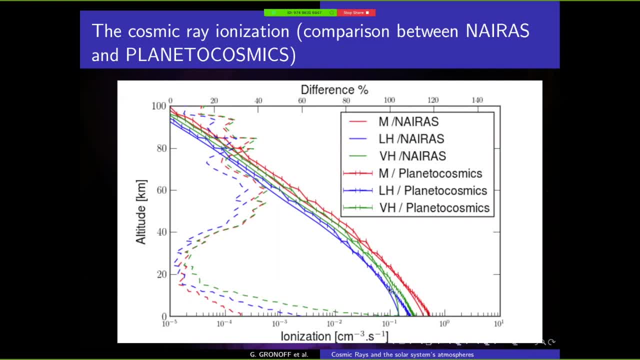 And you start to be to go to 60 to 80% difference, And you start to be to go to 60 to 80% difference, And you start to be to go to 60 to 80% difference. 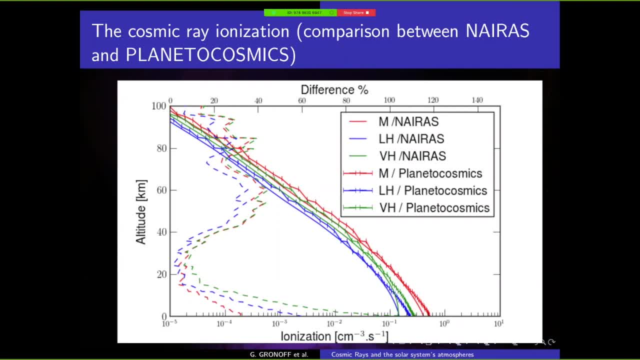 For some of the higher mass. So that's where we need to do a little bit more work to understand what's going on over here. We have a good theory of why it's different here, So we are working on it and it should be better. 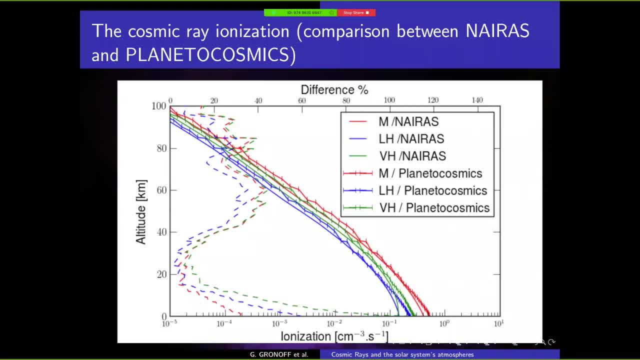 But what is important to understand here is that this doses have to be really close to each other, And when we start to work with NASA, when we start to work with people doing human safety, when we start to work with people doing human safety, 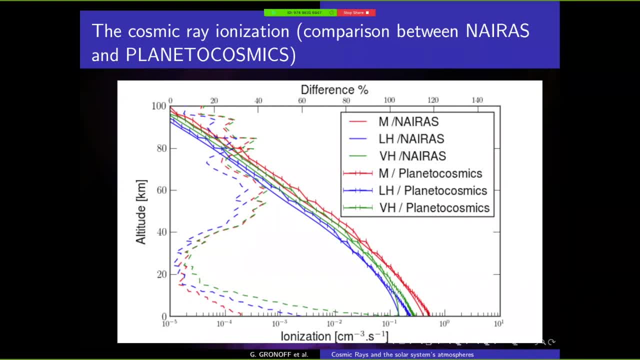 they have very high standard for the uncertainty and for the way we compute this and for the way we compute this, this values. So it's a little bit more complex than just having an estimate with 100% uncertainty, Because when we do physics, 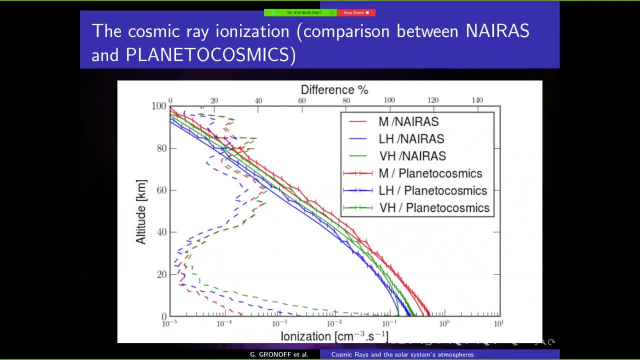 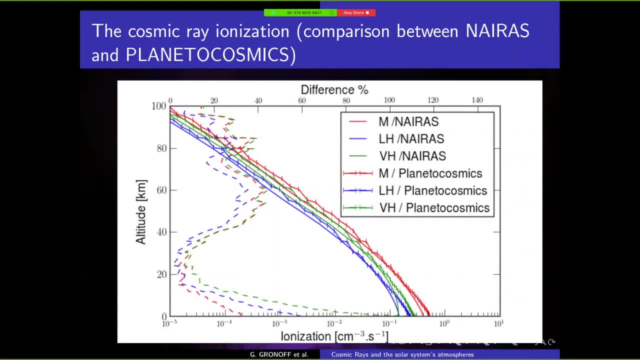 I am happy because I don't know how the. I don't know how the cosmic value in time really. I don't know how the cosmic value in time really. there is a lot of uncertainties about those factor. So having a big estimate of what's going on, 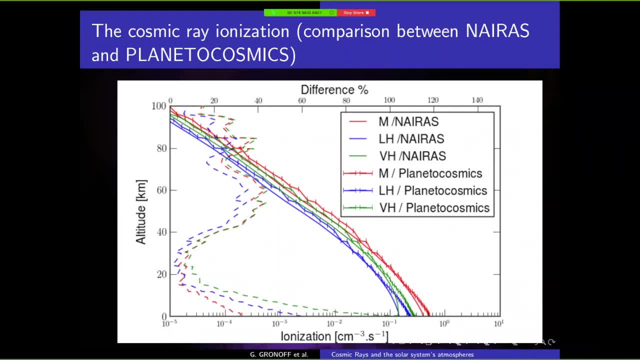 with a factor of 10 is great In human radiation safety. you don't want a factor of 10.. That can be the difference between I can go out safely and I am in a risk, in a high risk, and I am in a risk in a high risk. 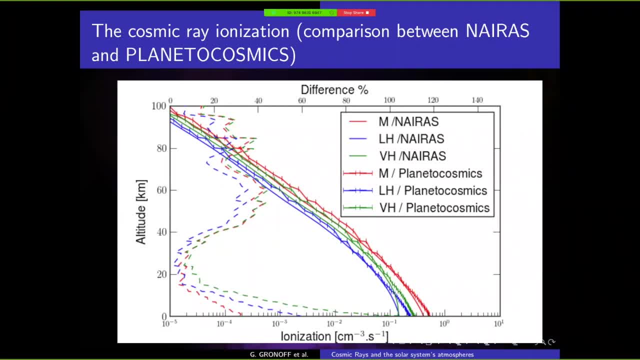 So that's why there is a lot of improvements, that is worked on all these codes. Okay, okay, Thank you, Thank you. Can I ask another question? Sure, So these models you have, NERAS and PLANET COSMICS or whatever. 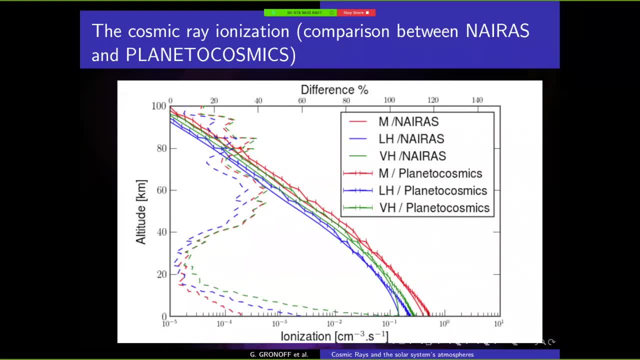 they're all the statistical right. They're statistical models, not predictive in the normal sense. I am not sure what you mean here. You don't predict an event, but you sort of predict their statistical behavior. Yeah, I'm predicting those from past events, basically. 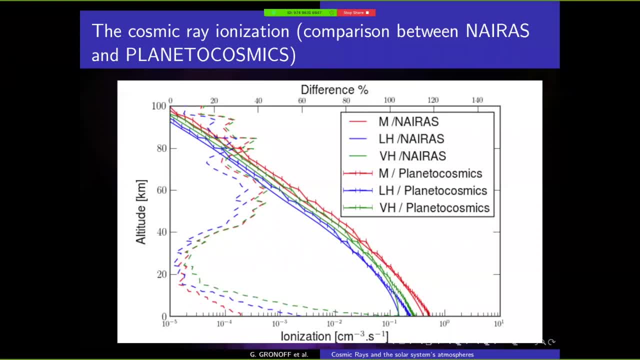 So there is a little bit of. it's a little bit different with NERAS right now because NERAS is an operational now casting model. It is looking at the current situation as a sun and tries to see what's going on. 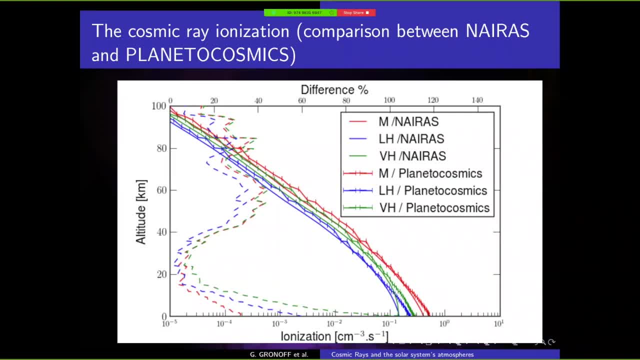 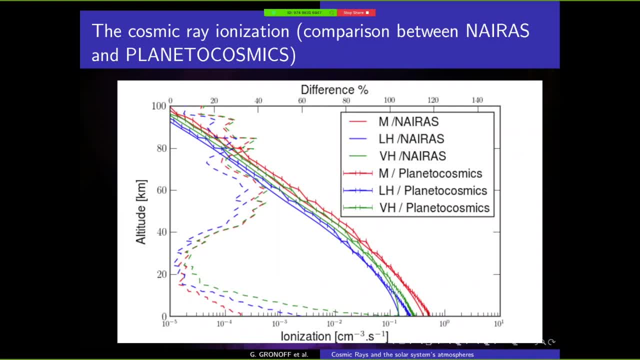 We have plans to try to use some of the predictive model of SCP event with NERAS. But all right, that's for now. with SCP event there is still a lot of uncertainty, but Okay, okay, Thank you. 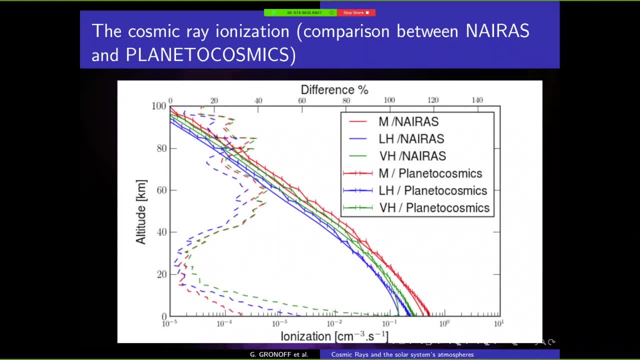 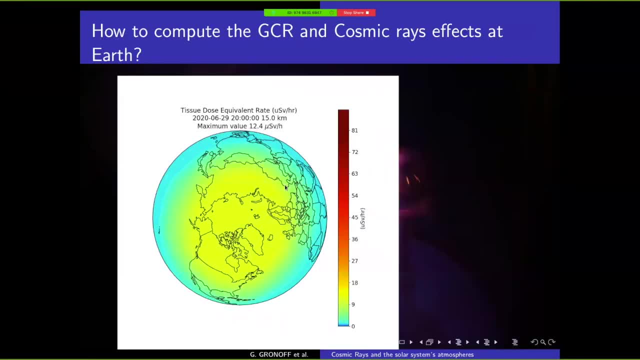 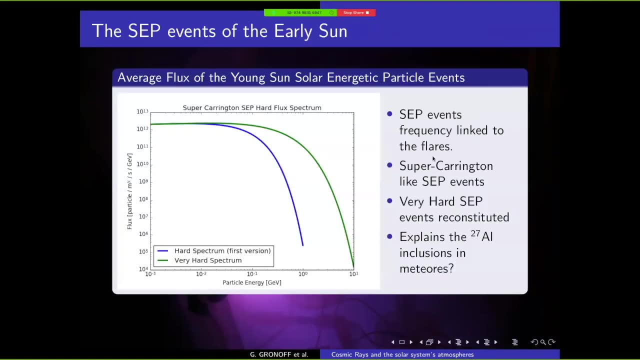 Yeah, yeah, Yeah, I had a question. So in one slide you showed that for early solar system you had hard spectrum pieces, events. So how did you calculate this? Wow, Yeah, Okay, so that's the work of Vladimir Hapetian. Actually, he has a couple of papers lately and I can send you the data on that. 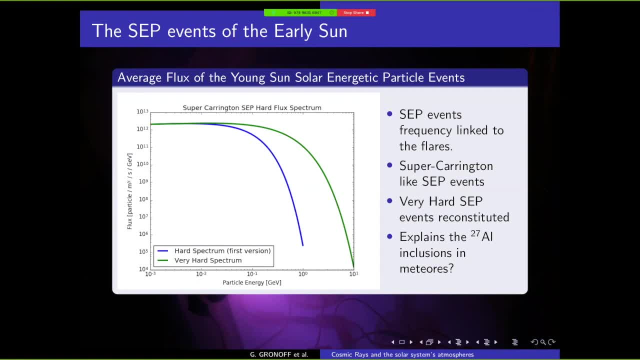 But so it's based on analogies with other stars. On the Kepler data, they look at young G-stars and they were able to look at the frequency of the flares on these young stars. Based on that, they have a lot of very 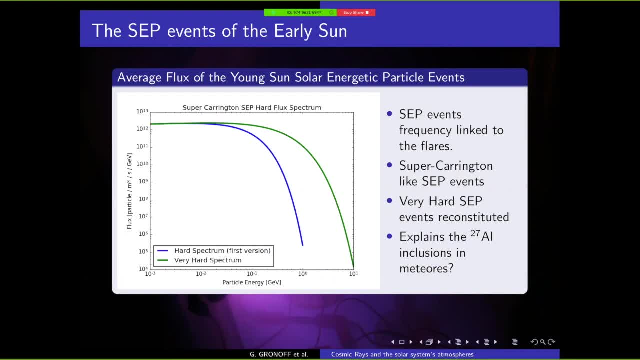 of statistical ways to see the probability to have SCP events And from this probability that are way higher. because it's basically what it is saying is that you have an SCP event of a kind of class every day or every two day, And from there they were able to reconstruct. 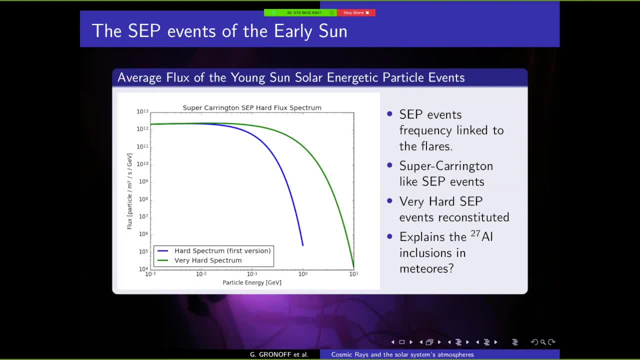 this flux and have an idea of what it was in the past. In addition to that, and that's really the latest of the work, they have models of how an SCP is produced And they are trying right now to reconstruct in a more physical basis this spectra of the young sun. 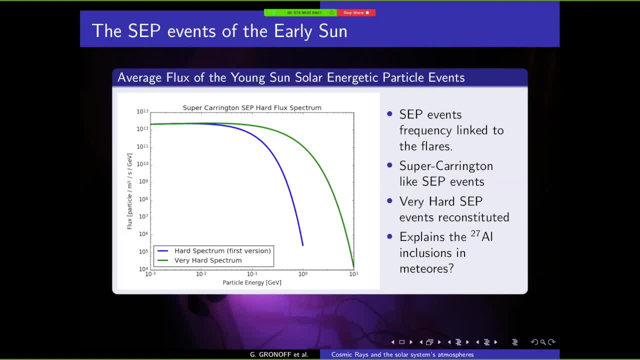 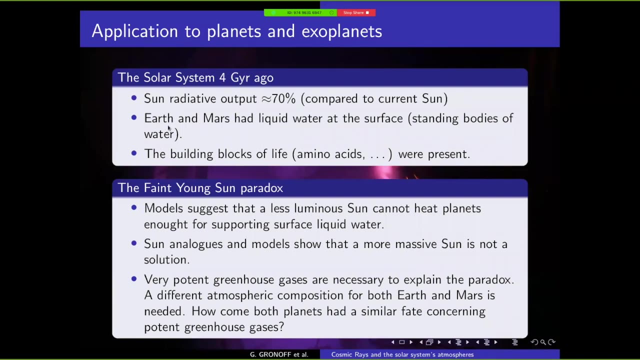 of the SCP events. All right, well, thanks. What is the Fein-Youngson paradox? What is that? Okay, so, yeah. so, basically, when you look at the Sun, you see that it changed its flux, its visible flux, the IR flux.